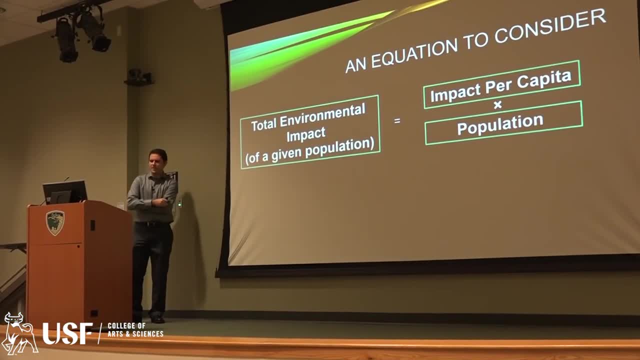 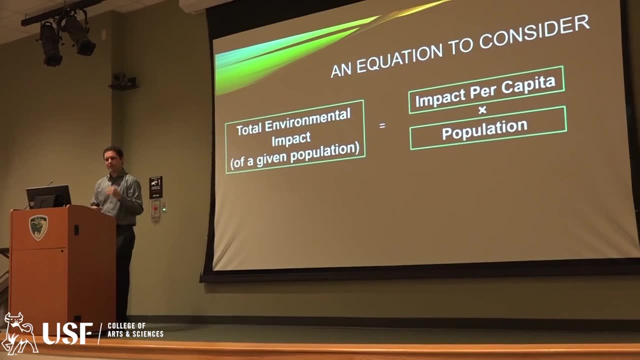 We'll do the equation first. The equation is pretty simple. It's an equation for total environmental impact And I'm breaking it down just to two variables. Now you may see others. there's a common one known as IPAT, which takes environmental impact to be a 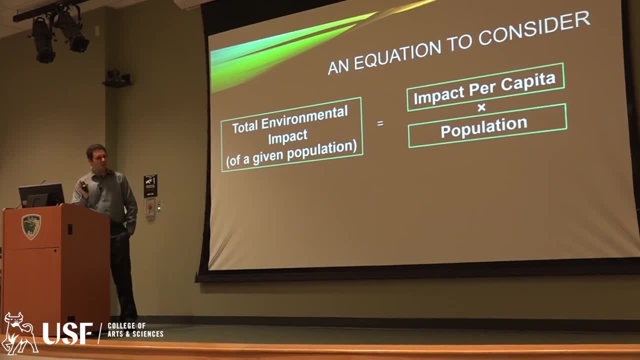 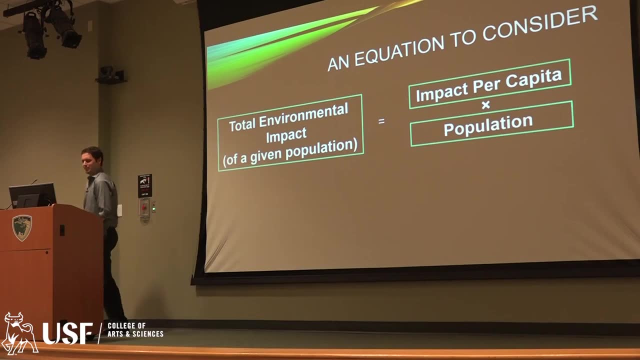 combination of population affluence and technology. I don't like that equation as much because affluence and technology are kind of common. It's complicated to assess And I like to have simple things to work with when we're looking at these sorts of problems. Technology, for instance, can function as both a way to 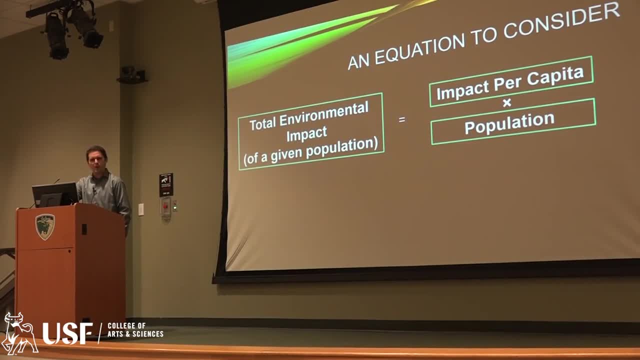 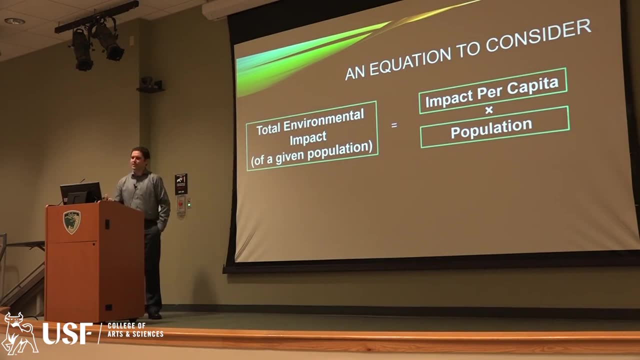 reduce environmental impact depending on which technology is being used or a way that increases it. And I like to think of it more as two different forces: average impact per capita and population size that multiplied together give you total environmental impact of a given population. 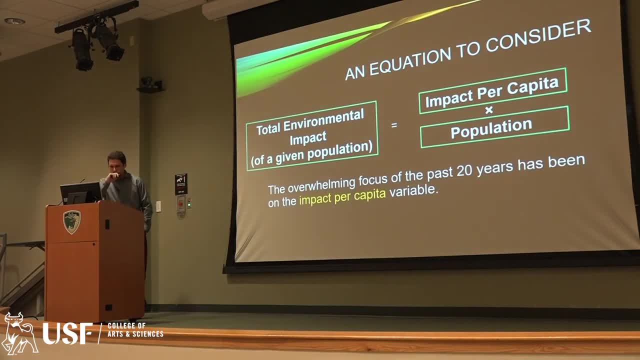 Oops, my pen. There we go. So at least in philosophy- and I get the impression this is true across other disciplines as well- the overwhelming focus of environmental ethicists has been: how do we reduce rates of environmental consumption, especially in the Western world where we consume depending? 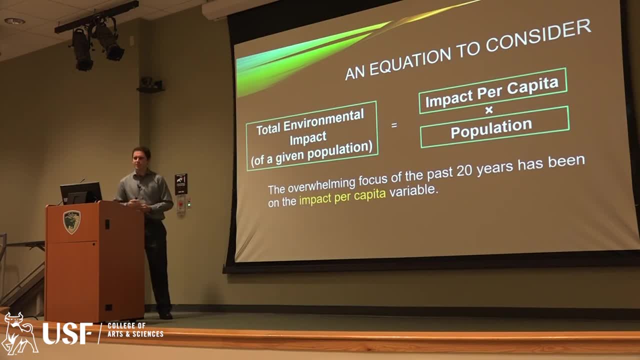 on the country, especially in the United States, 15 to 20 times the resources of people in certain parts of the developing world. It seems like that's the main source of our problems, whether it be climate change, resource depletion, species extinctions, etc. Whatever it is it. 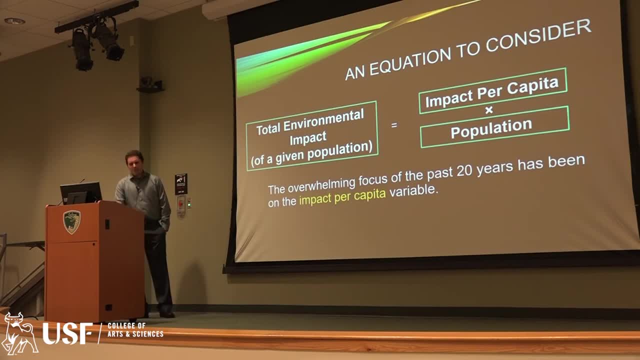 seems like that's the main culprit, And there is some truth to that. Everybody who works on these issues agrees. reducing impact per capita, reducing our average rates of consumption, is really, really important. What I want to suggest today is that we also need to be looking at the other variable. 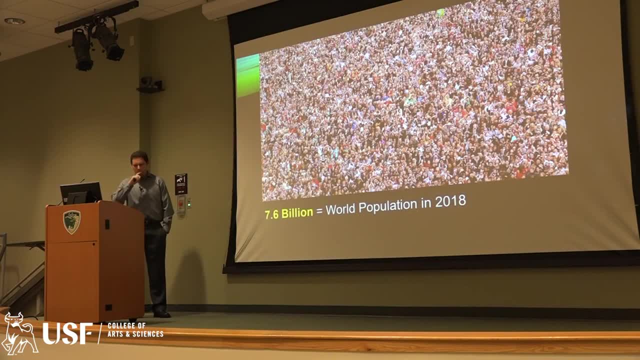 and then I'll talk about some ways we might do that. So here are the numbers I alluded to, The 7.2 in particular: One is 7.6 billion, the other one is 11.2 billion. The 7.6 billion. 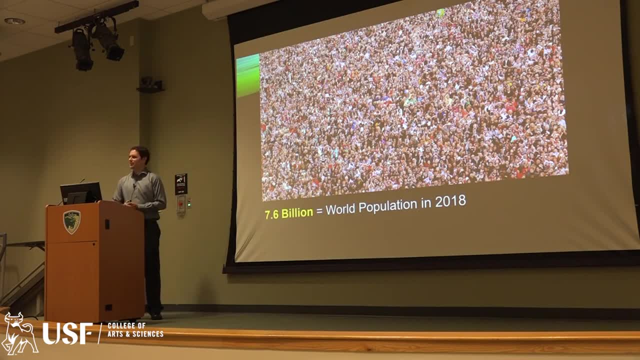 is how many people there are on the planet right now, by our best estimates. The 11.2 is the UN's projection for how many people we will have in the world in the year 2100, according to their most recent estimates that were conducted in 2017.. 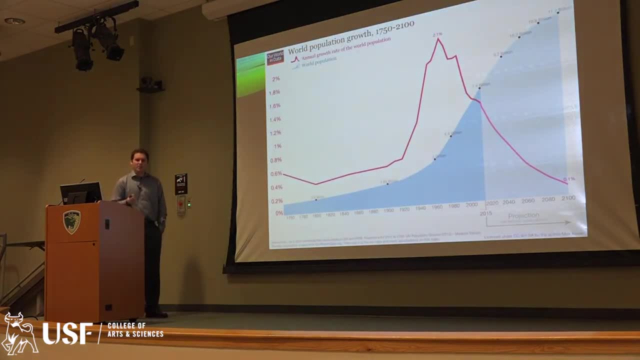 Now to put this in perspective: if you go back to about the year 1800, we didn't even have a billion people on the planet yet. So in just two centuries we've gone from crossing the 1 billion threshold to crossing the 7. 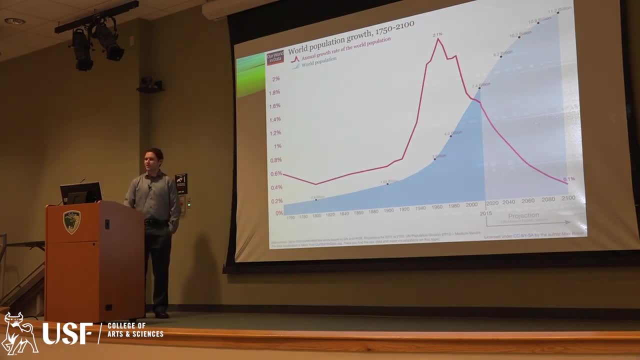 billion threshold and by the end of this century we are projected to cross the 11 billion threshold. So we're looking at a massive increase in global population in a relatively short period of time. Now the other line on this graph beside the number of people on the planet is: we're looking 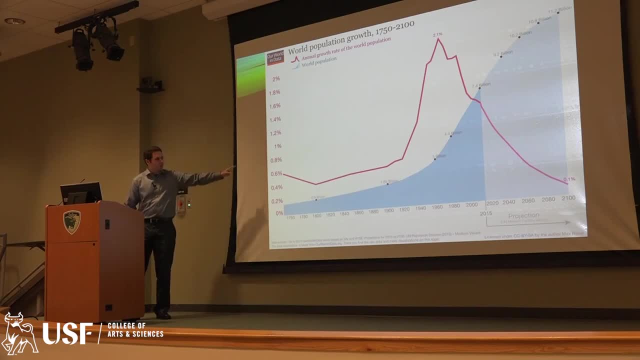 this blue graph represents population growth. The red line represents essentially the percentage increase of population growth per year. One misconception a lot of people have about human population is that the problem is going to solve itself because, as you can see, the population increase percentage-wise keeps going down, or at least it has been. 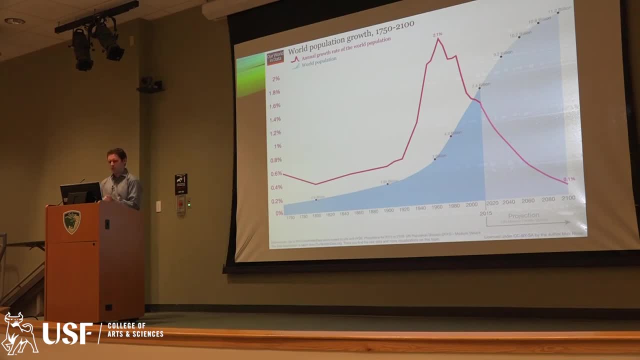 since it peaked somewhere close to 1970.. I can't remember the exact year, but I want to say 1967 was the actual peak year. But it's been going down steadily since then. but the problem is the total number of people has gone up so much. 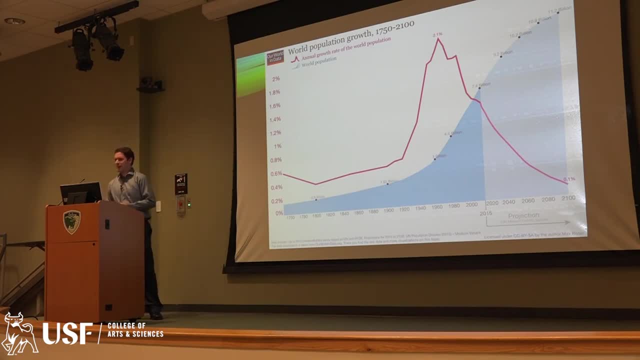 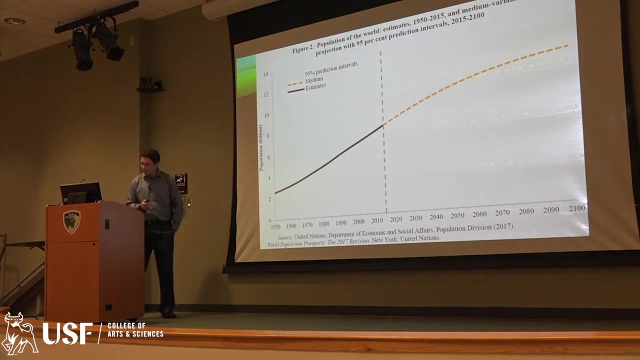 that, even though the percentage increase has kept going down, the total number of people that get added every year has stayed almost the same. About 70 million people added to the planet total every year. Now the projector here has diluted their 95% confidence interval. 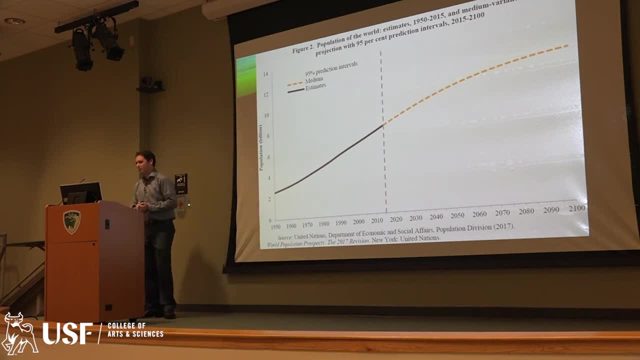 This is a sort of measure of the UN's estimates for where we wind up in 2100.. The end of that dotted line corresponds to roughly 11.2 billion people, But there's a 95% prediction interval that goes as high as a little over 13 billion. 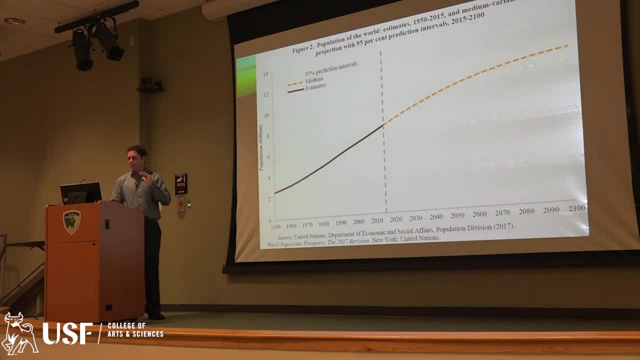 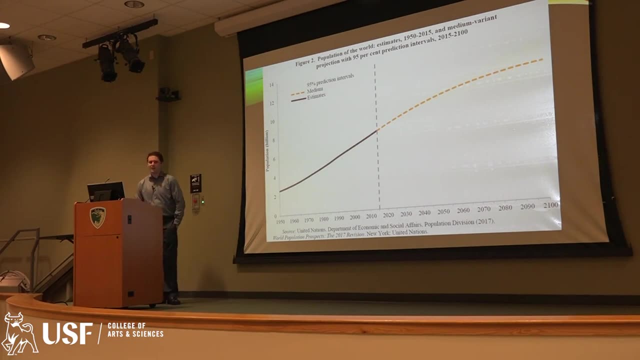 or as low as about 8.9 billion. So there is a potentially huge range. There is a great degree to which we could affect how many people exist In the year 2100.. But their medium range variant, their sort of moderate prediction, 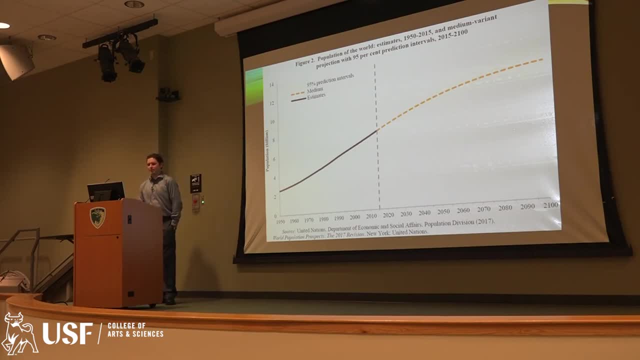 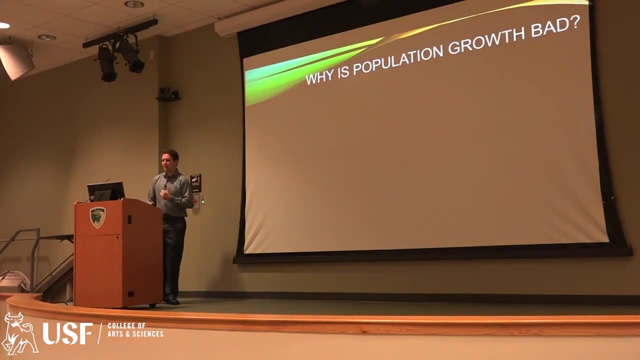 puts things at typically about 11.2 billion. So why is it that increase in human numbers is bad? Well, the first thing I want to say is it's actually not bad in itself. It's not the case that just because someone new comes into existence, it automatically follows someone else. 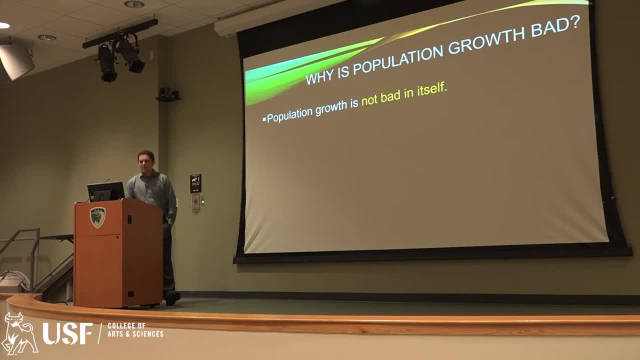 must be worse off in the world. Rather, population growth in this context is bad because of all these different environmental impacts that we have that it contributes to, And I'm not going to focus on every single one because our time here this morning is finite. 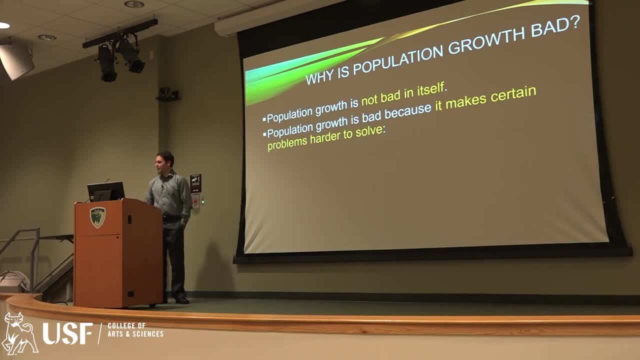 I'm just going to highlight four of the most significant and the most commonly mentioned ones in the literature. So food shortages, water shortages, species extinctions or biodiversity loss, as conservation biologists often say, And, of course, climate change, which is perhaps the big one, if there is a big one on this list. 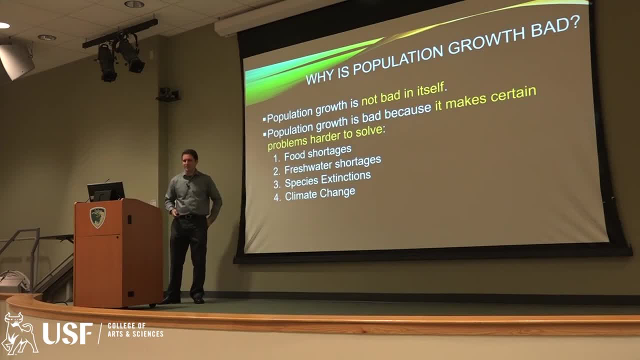 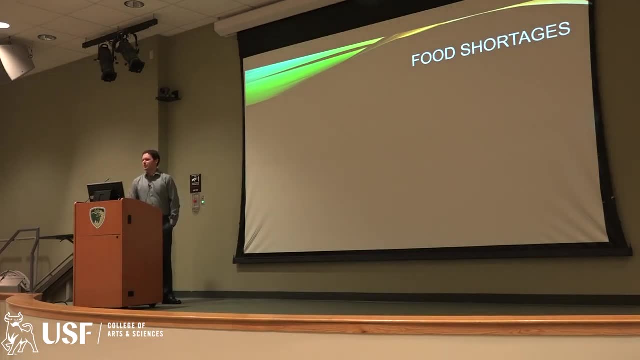 Because climate change itself will affect all three of the others as well. Now, food shortage is an interesting one because, if you look at the history of discussions of populations, this is what people will bring up. Economists love to point out the fact that the two people who are more likely to die from hunger and hunger are people of color. 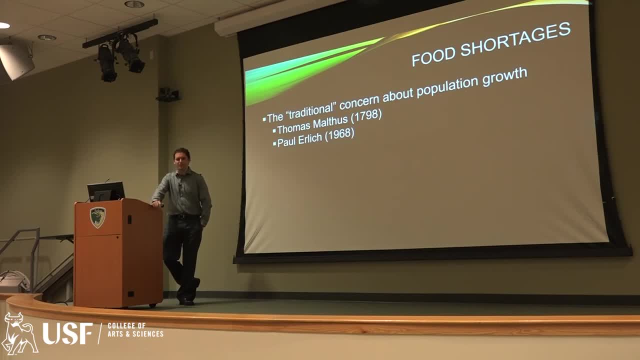 who predicted population related catastrophes. Thomas Malthus and Paul Ehrlich were wrong in their predictions, in their assessments of what was going to happen. In both cases they predicted massive food shortages would result from increased population growth, basically from just population rising so rapidly that global food supply couldn't keep up. 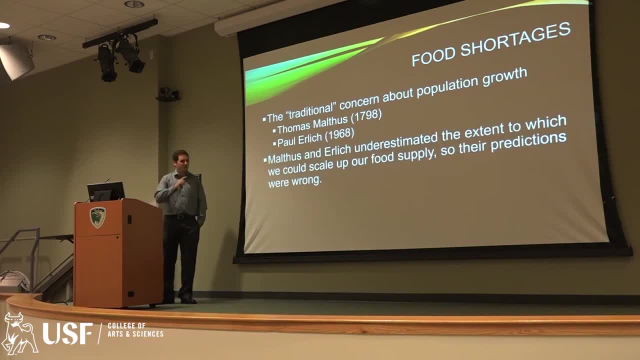 And in both cases they were wrong. And they were wrong for a particularly straightforward reason: They just underestimated our ability to scale up agricultural production. They underestimated our ability to come up with technology that would improve our agricultural output. So the reason I highlight this is because there's a tendency for people to think that, because 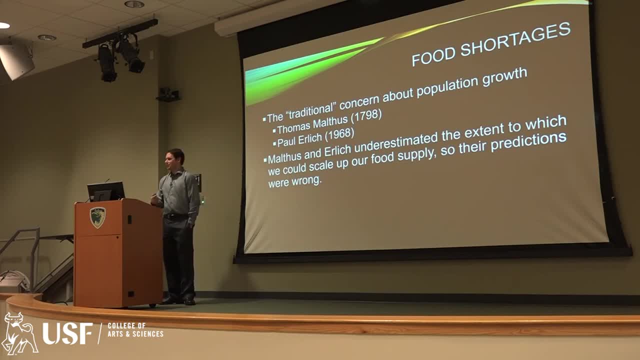 Malthus and Ehrlich were wrong about this, that it follows that any serious concern about population in the future will also be wrong, But I think that's a mistake. So let's talk about what our situation is in 2018 with respect to food shortage and these other issues. 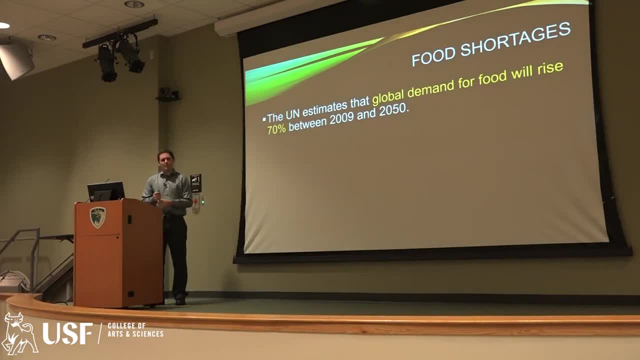 So the UN estimates that global demand for food is going to go up from relative to 2009 levels by about 70% by 2050.. Certain other people actually think that those estimates are kind of modest. So Sarah Menker, who runs an agricultural data company, for example, has a. 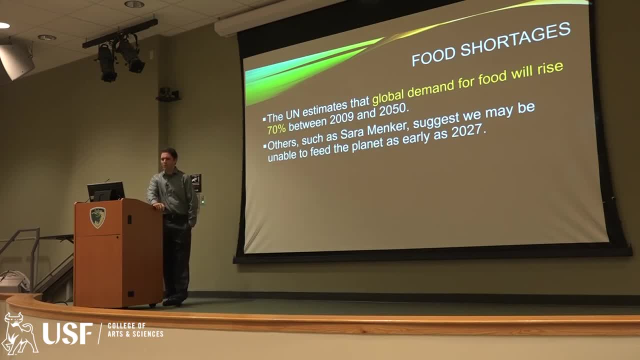 recent TED talk where she argues that we might start to run out of food if we were to distribute the food. even if we distributed it perfectly and equitably around the world, we still wouldn't have enough people enough to feed the world. She thinks that might happen as early as 2027.. The most common estimate, though, is still the UN one. That's what you'll see if you look this up in the literature. We've got to find a way to increase food production by roughly 70% to meet demand by 2050.. 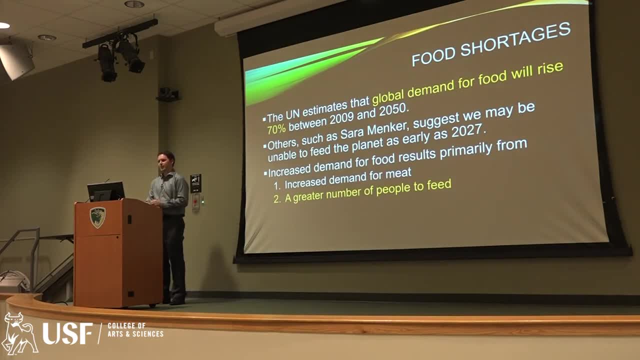 There are two factors that contribute to increasing global demand for food. One is an increased demand for meat. That might not be super obvious, but that's one of the factors. So the basic idea is, if we're going to raise cattle and sheep and pigs, chickens, etc. you've got to feed them. 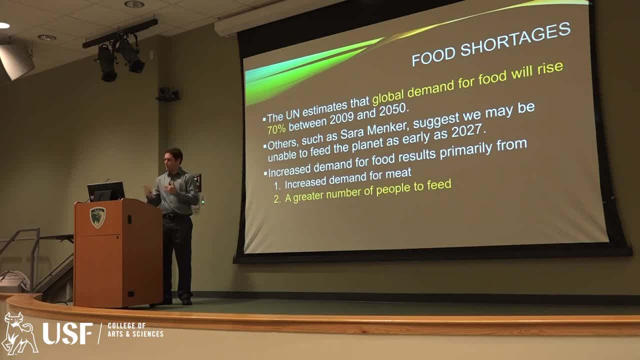 And so instead of growing grain, for example, to feed two people, you are instead feeding it to livestock, And then the livestock are later consumed by people. But in this process a significant amount of fish cheese is being produced. significant amount of the processes is, just from a calorie standpoint, much less. efficient. it would be more efficient for humans to eat that grain directly rather than raising livestock. so as you scale up meat production, you have to produce more food overall than if you have a strictly vegan or vegetarian diet. the other thing, of course, is the other factor. there are just more people there. are just more people to feed. other things equal. a population of 11.2 billion is a lot harder to feed than a population of 7.6 billion. another thing worth pointing out is these kinds of estimates operate in sort of an idealized world, a world we do not live in. in 2016, there were roughly 800. 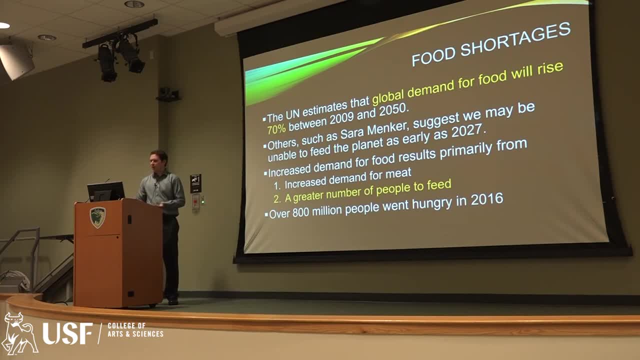 million people on the planet who went hungry. the reason why is because, even though we technically have enough food to feed everybody in the world, various social and political realities prevent it from being equitably distributed. you can't feed everybody in the world. you can't feed everybody in the world. 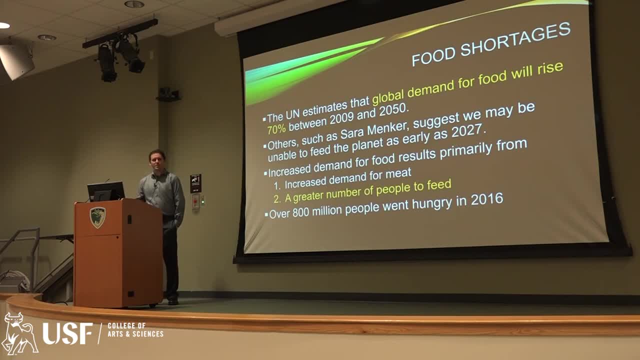 and so you've got lots of people in various regions that still nonetheless starve or live in conditions of more or less constant hunger, even though it is theoretically possible to feed them. so I would expect, if we indeed don't even have enough food to meet this global demand in 2050, it's not the case that 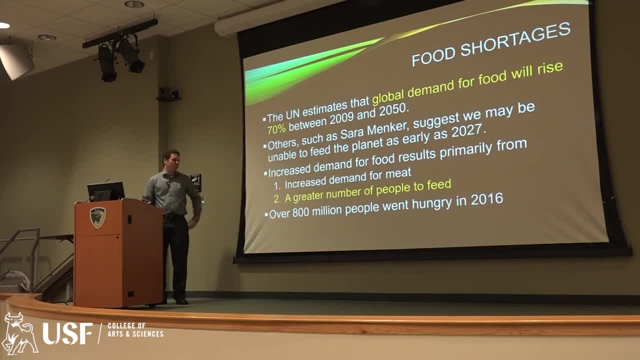 we'll see a small number of people who we can't feed. we'll see this number go well above 1 billion. it's not going to be a good thing if we don't have enough food to feed everybody in the world. we're not going to be. this isn't going. 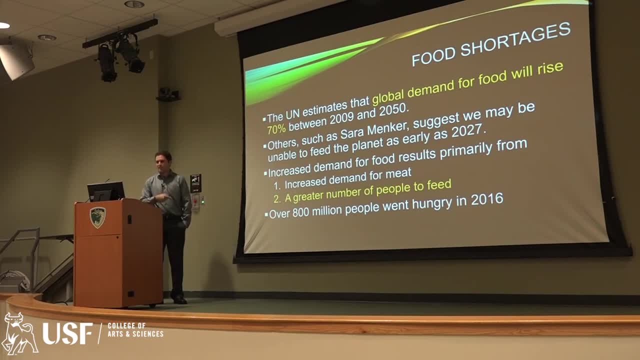 to be a case where we're going to magically solve those problems of food distribution in the next 40 years. we should expect that they're going to continue and so we should expect that this number will be even more, will be even, will rise even higher than its current amount. 800 billion is already a 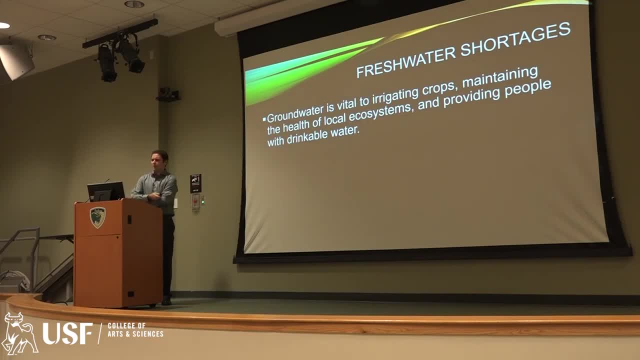 lot, that's over 10% of the people in the world. another one that comes up is fresh water. I'm going to focus particularly on groundwater, because it will. you need groundwater for things like irrigation, maintaining the health of local ecosystems and, of course, providing water for people to drink now. 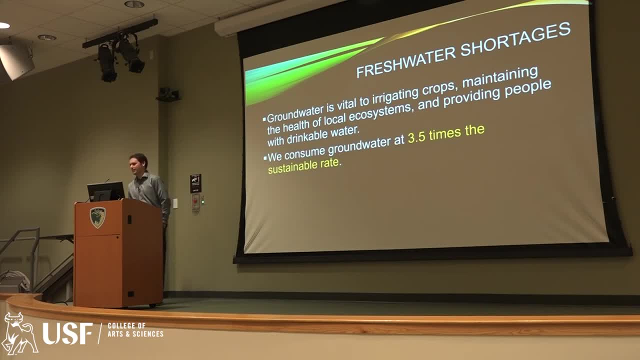 groundwater is a renewable resource. it replenishes itself over time, but not it. if you consume it too quickly, it doesn't replenish fast enough, and so the situation we're in right now is we are consuming groundwater worldwide at roughly 3.5 times the sustainable rate. so if we keep doing that, eventually 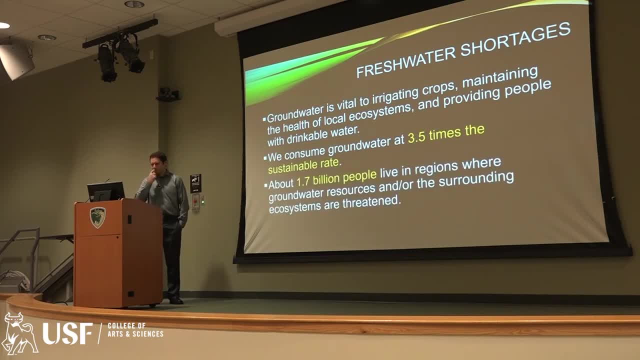 we're going to have significant short-term. in various parts of the world there are 1.7 billion people who live in regions where the groundwater resources or there's, or the surrounding ecosystems are threatened in some way. so if you scale up the population in these, 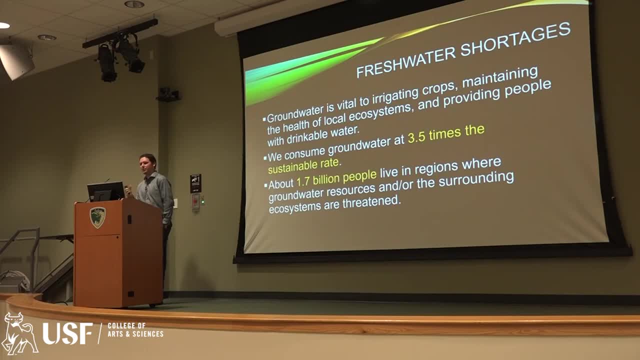 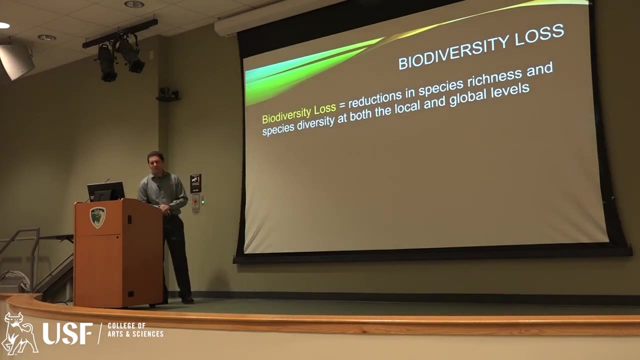 particular areas, those that problem becomes even more intractable. it becomes even more difficult to reduce your rate of groundwater consumption to a sustainable level. this is species extinctions or biodiversity loss. the way I'm defining biodiversity loss essentially in terms of reduction of species, either in terms 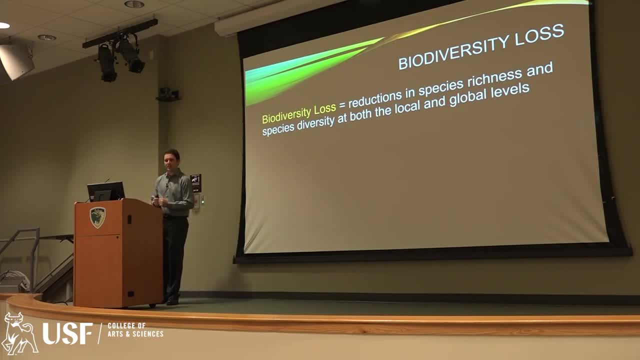 of their richness, or just their, in other words, their population number in a given area, or in terms of their diversity, which is what would be affected if species actually went extinct. you can have biodiversity loss locally, in different regions. you can also have it globally. the biggest reason why we're in 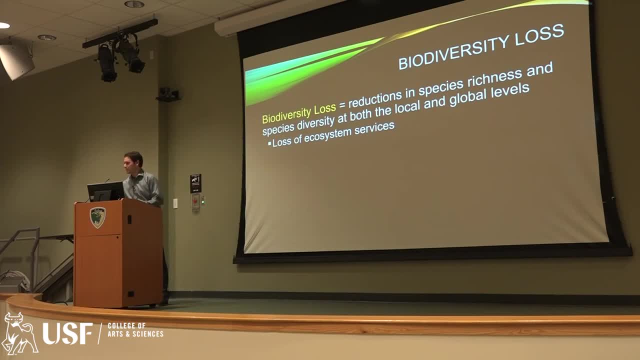 this situation is because it results in a loss of biodiversity. loss for human beings is because it results in a loss of ecosystem services. ecosystem services, or a combination of functions of ecosystems that provide resources to us at very, very cheap economic costs. in some cases, the resources that are 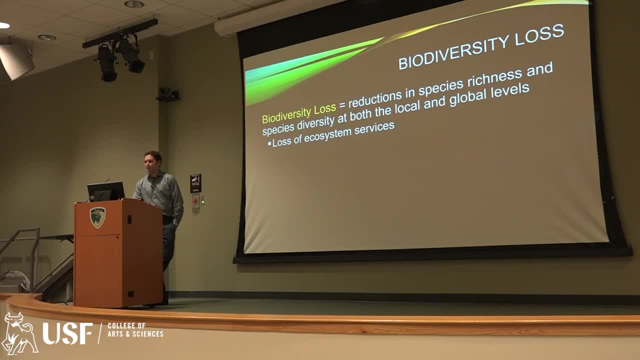 produced would be either too costly or simply impossible for us to produce ourselves. biodiversity loss also results in a loss of compounds that we can use to make medicines, so there's a pharmacological component here. so you, if you get more and more species extinctions, particularly of plants, you, 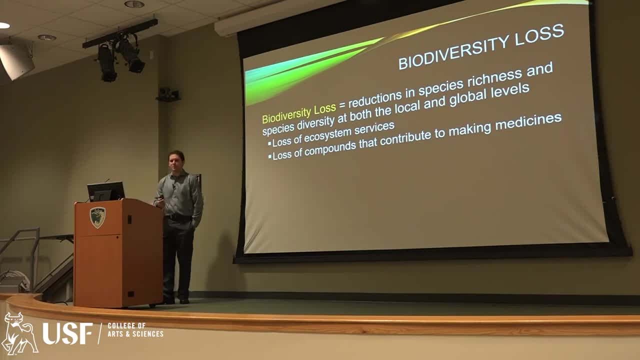 lose a resource that you can use to make medicines that contribute to alleviating various human ailments. another concern is epistemic, or knowledge-related. so EO Wilson has pressed this point rather thoroughly. views. you know, every species on the planet is a certain source of knowledge. 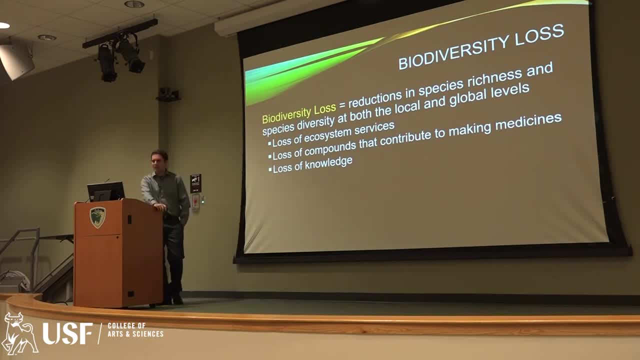 about our world and about how best to interact with it. you lose a species from the world and you essentially lose a deep resource of knowledge. the other big one and I don't, I don't know. this kind of depends on the species. some people really, really like polar bears. 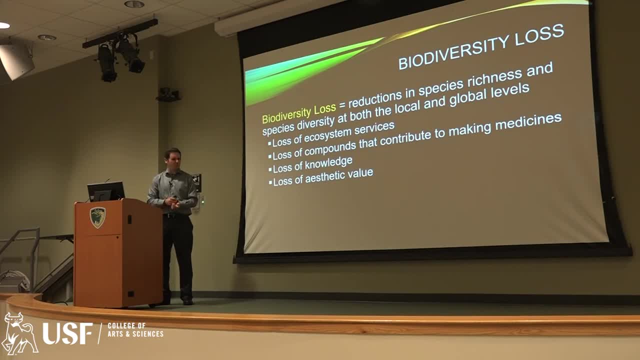 for example, or pandas less concerned about, say, the salamanders that live in the Great Smoky Mountains. all these species are threatened. some species carry a kind of aesthetic value that people really care about. of course, that aesthetic value doesn't always have to just be just be beauty or that kind of charisma that some of these animals 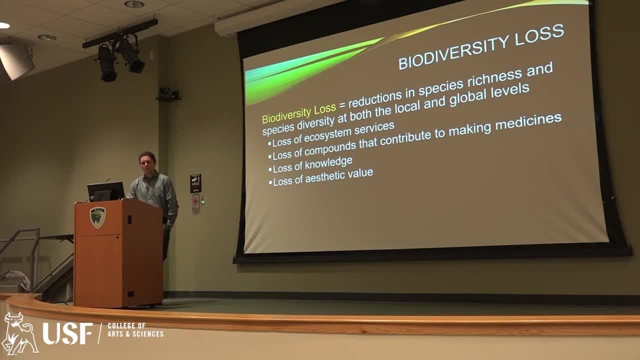 have. it can also just be kind of a sense of wonder or perplexity, but in any case you lose a species, you lose a source of real-life aesthetic value. so for all these reasons and few others, conservation biologists are deeply concerned about the rapid species extinctions that we're seeing. you might 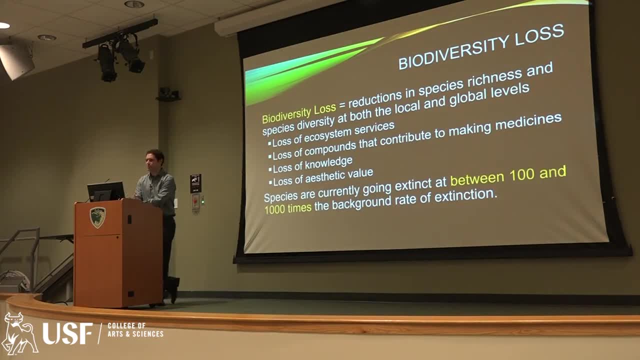 wonder exactly how bad that problem is, because, of course, species do go extinct naturally in the world at a certain rate. the issue is that, based on, depending on which estimate you cite, we're currently seeing species extinctions at roughly 100 to 1,000 times the background rate. 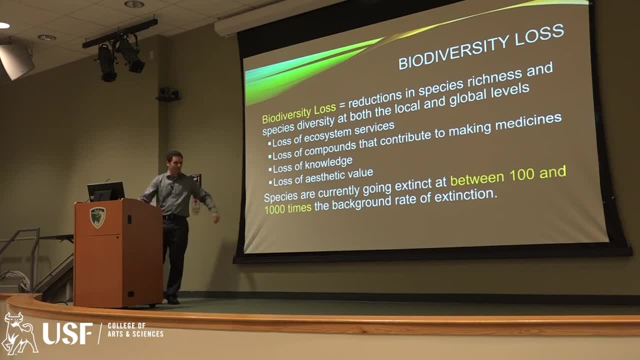 and obviously that's a huge range. the most recent stuff I've seen is closer to the 1,000 number. in the past, the most common estimate has been about 100. I don't think it really matters which one you think is correct, because either way 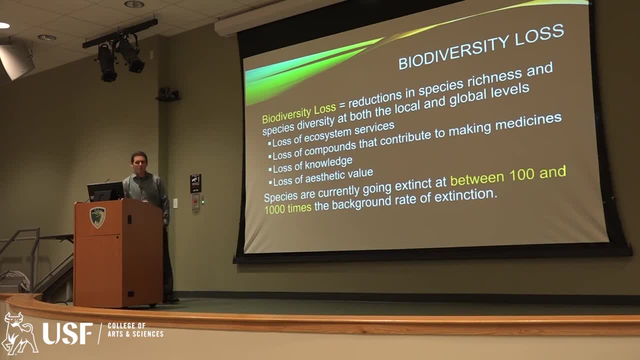 that's crazy. that is an extraordinary effect. I mean, the background rate of extinction is designed to be an estimate of how fast extinctions occur in the absence of human activity. so how many extinctions where we're seeing before humanity showed up on the scene, and so for us to be impacting non-human life to this. 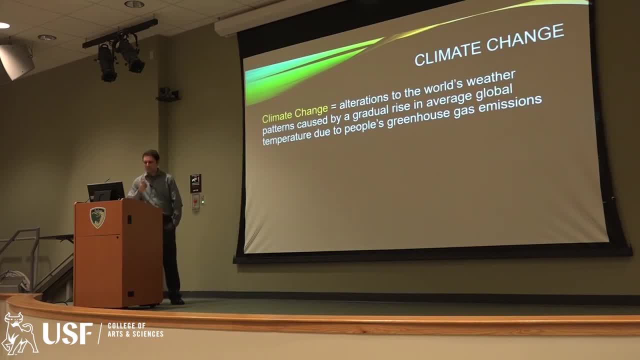 extent is rather extraordinary, and I've saved the biggest one for last because, as I said, climate change affects all the other issues on this list. what I mean by climate change- I hope this is a pretty common, agreed upon definition- is alterations to the world's weather patterns caused by a gradual rise in 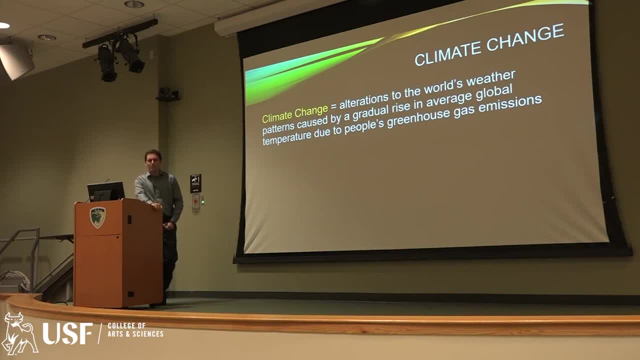 average global temperature due to anthropogenic greenhouse gas emissions, or in other words, human-caused greenhouse gas emissions. So again, it's not a complete list of effects, but these are all really well documented. You can read the reports of the Intergovernmental Panel on Climate Change to get the low. 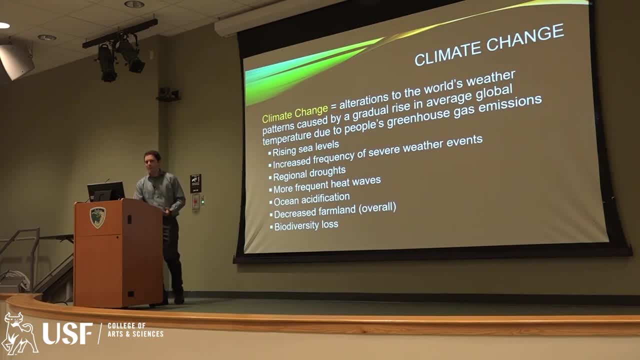 down on all this stuff. What do we expect from climate change? Well, we expect sea levels to rise, which will displace hundreds of millions of people around the world, make certain areas uninhabitable or unlivable. We expect increased frequency of severe weather events. We've already seen some. I've only 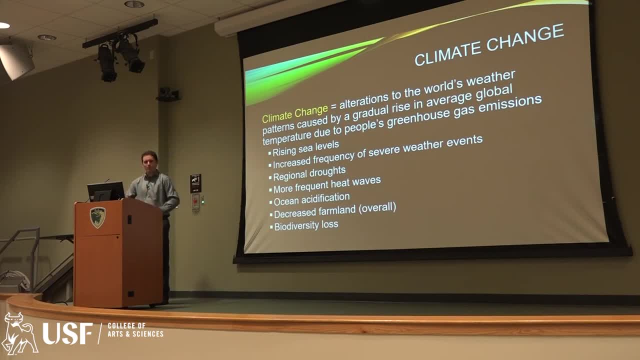 been in Florida for like 14 months and already it's been hit by two huge hurricanes. We should expect those kinds of events to become more common in the future because, as we move forward, we're going to see more and more and more storms. We should expect more regional droughts, because there will be more 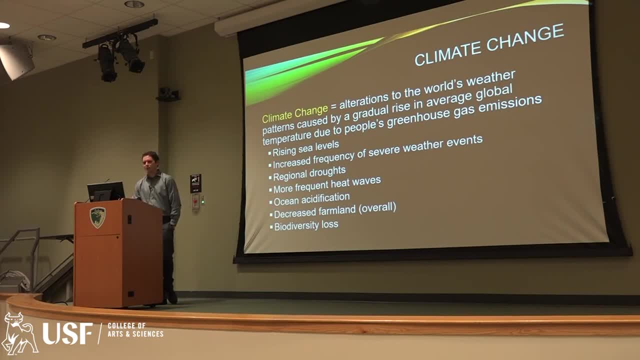 common heatwaves. This is one way in which water shortage can be contributed to directly by climate change. We should expect ocean acidification, which is a significant source of biodiversity loss for marine life, And, interestingly enough, farmland will be affected asymmetrically around the world. 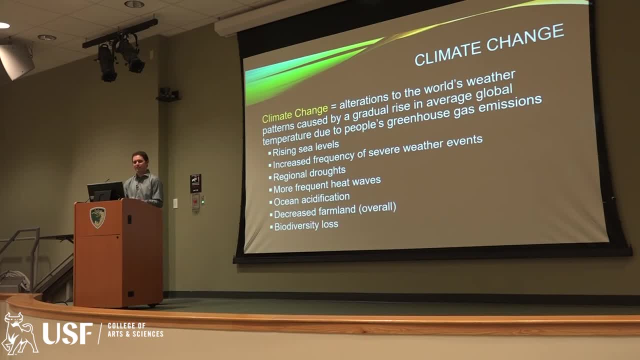 If you live in Siberia you actually might see more farmland than you had before, But overall, worldwide there will be a reduction. Part of it because of sea level rise, which will essentially make certain areas near coastlines that used to be farmable land no longer farmable. 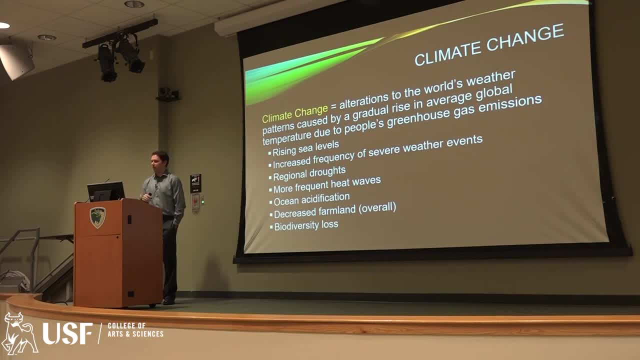 but also, just as regions near the equator become more arid, you won't be able to grow crops nearly as easily there as you could before. And the other one, which I just mentioned, is climate change also contributes to species extinctions, because some animals cannot survive in environments that are outside of a certain temperature range. 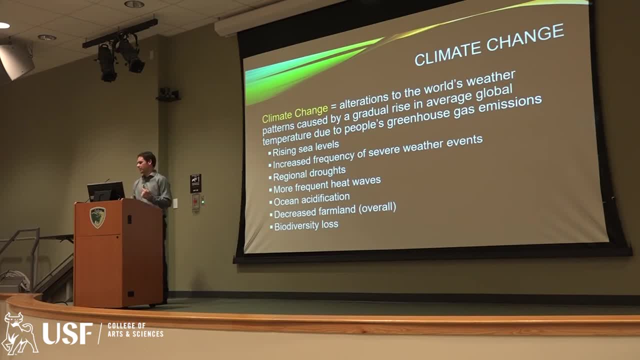 And so they wind up either trying to migrate toward the poles to get away from the rising temperature, or they go up mountains. The problem is that in some situations, like if they're living on an island, for example, they can't do that. 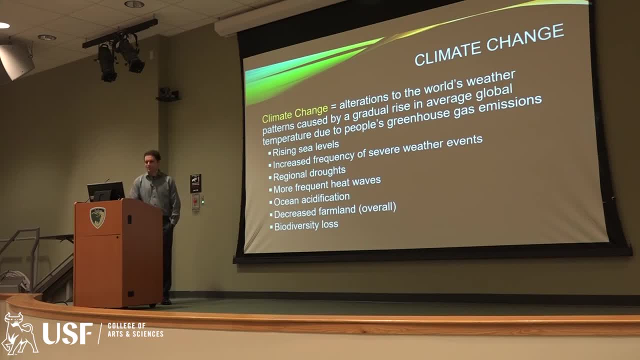 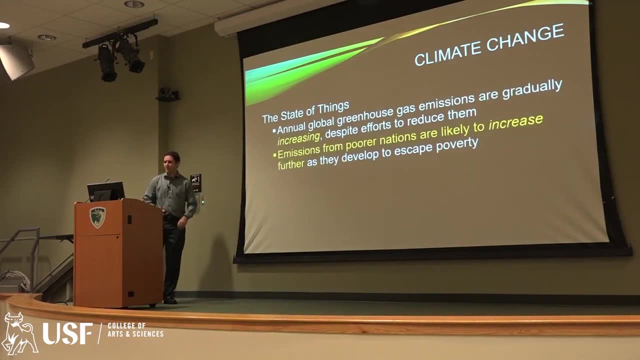 And so often they just get wiped out as a result of the temperature changes. Now, in climate change, there are two things that need to be stressed. The first one is, even though we've known about this problem for a couple of decades now, 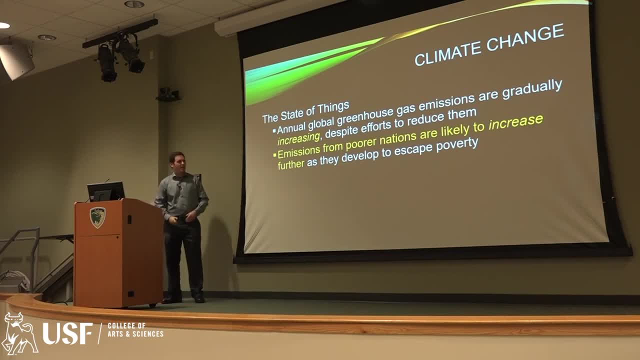 and been talking about it and making empty political promises. annual greenhouse gas emissions worldwide are still going up, And so we have not yet succeeded in even reaching the peak in terms of annual greenhouse gas emissions. We are still on an upward trajectory with those. 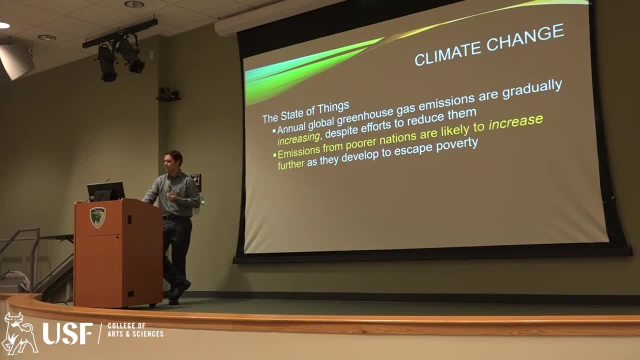 And in addition to that, in the near future we have to expect that emissions from developing nations will also increase More so, especially in China and India, because as these nations develop and as they try to lift their citizens out of poverty, at least under current conditions, that's going to require the use of fossil fuels to some degree. 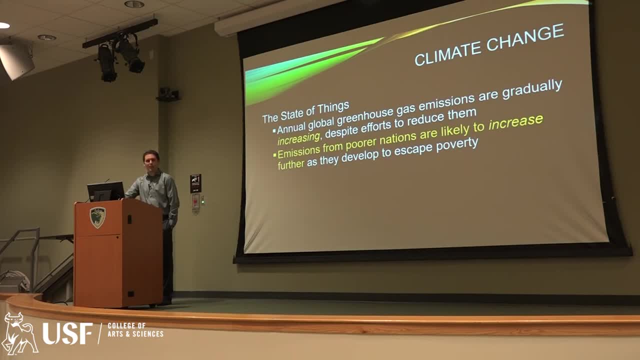 And a number of people have argued that these people need to be allowed to develop in that way, because in some cases their citizens are not even able to meet their basic needs. Their individual carbon emissions are almost perilously low. They are so low that the only way they're able to maintain those levels 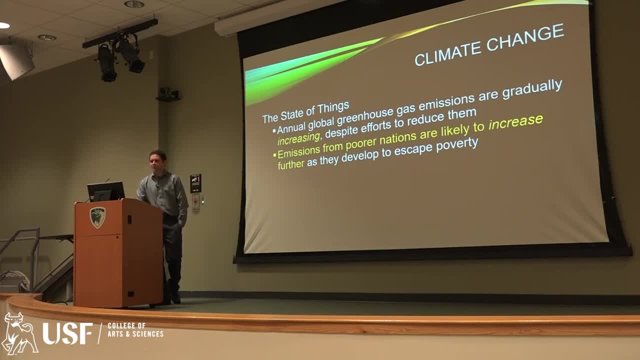 is by having tons and tons of people who are just barely even able to survive. And the thought is, if people like us can live very, very carbon-intensive lifestyles of luxury, those people should at least be able to emit enough carbon to meet their basic needs. 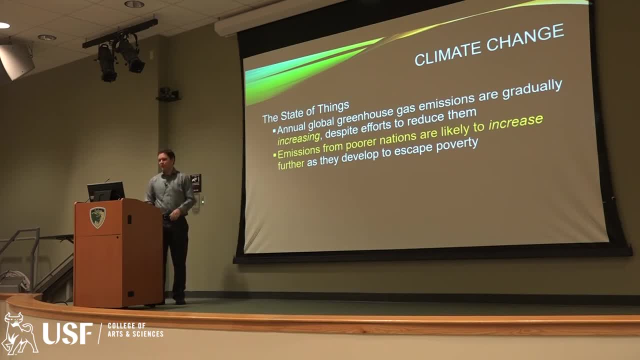 So the point between these two observations is: it looks doubtful that we're going to be turning the corner on climate change in the immediate future. I think that meeting the goal to stay below a 2 degrees Celsius rise in global temperature relative to pre-industrial levels. 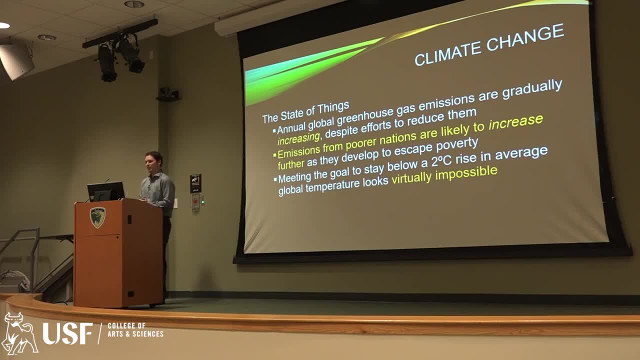 is the general goal that has been endorsed at a variety of these meetings and, as a part of the Paris Climate Accord that we are currently- the United States is currently in the process of trying to pull out of, I think meeting that goal has basically become almost impossible. 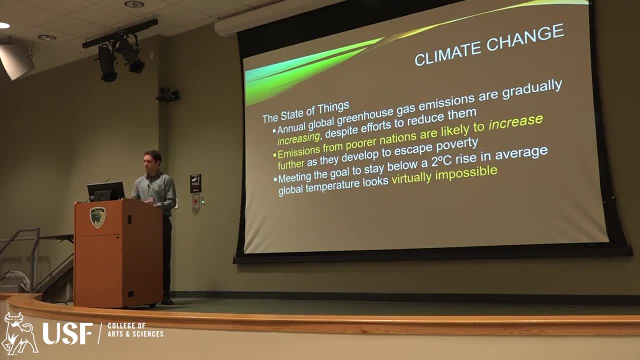 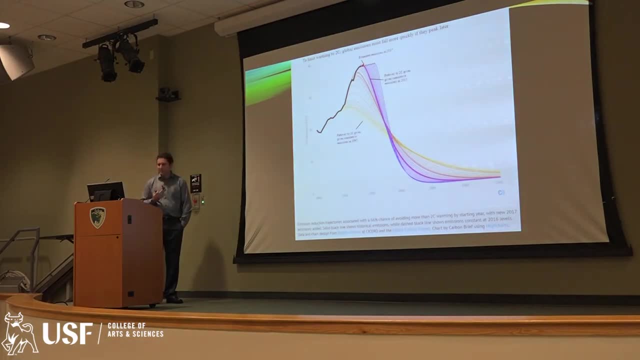 overlooking the possibility of radical and extraordinary geoengineering of the atmosphere in some way To give you an idea of how rapid the descent in greenhouse gas emissions would have to be to meet the 2 degrees C threshold. That red dot there at the very top is designed to be like where we are. 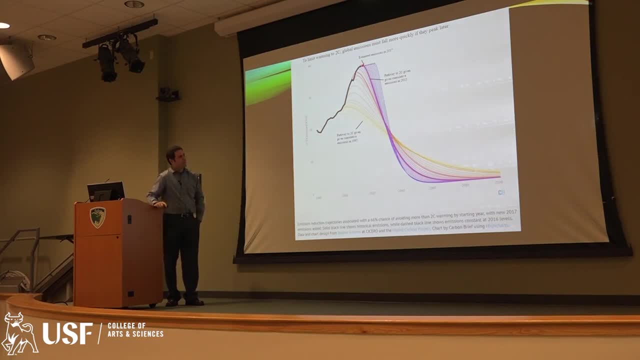 or where I guess we were in 2017.. And every year that you delay hitting your carbon peak and going down, the descent has to be a little bit steeper every single year. So even if we were to start right now, in 2018,. 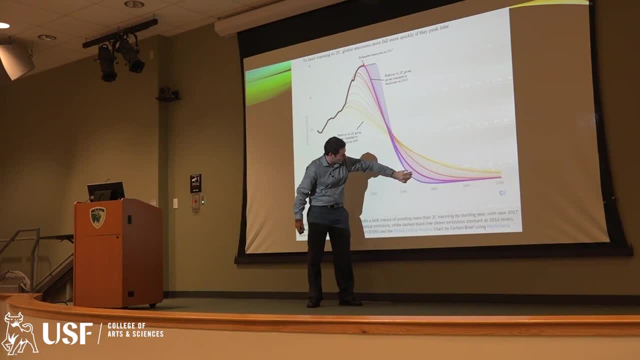 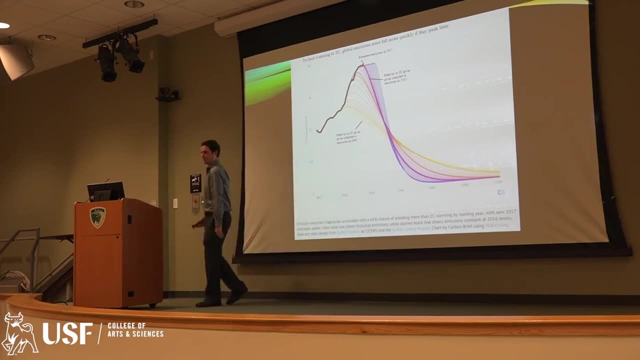 we've got to pull carbon emissions down by 2040 to roughly 5% of their current levels. That's impossible. There's no way that's going to happen And by the time we get to 2050,, 2060,. 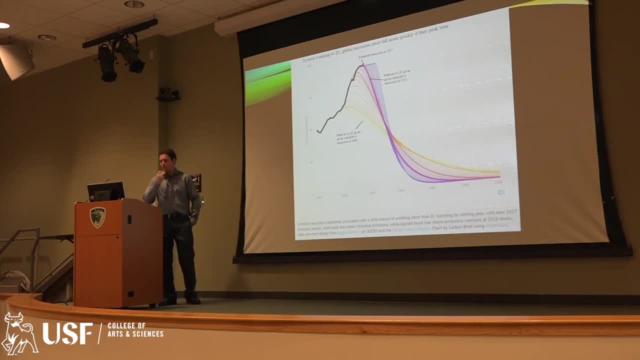 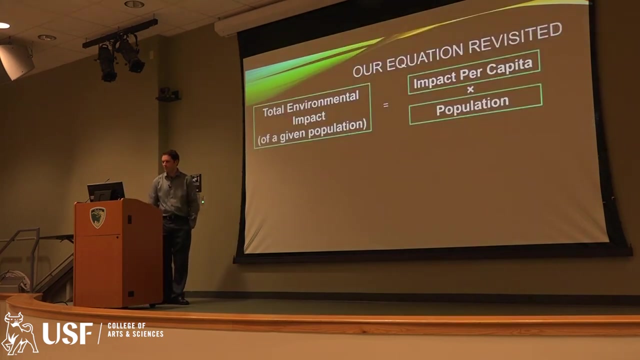 we'd have to be close worldwide to zero carbon emissions to make this sort of thing happen. There is just too much that would have to change socially, politically and economically for that kind of transition to be feasible. So let's go back to the equation here for a second. I mentioned this point earlier. I'm going to stress it again. I am not saying that reducing human numbers or stabilizing global population rise sooner rather than later is a panacea for all environmental problems, or that it is the ultimate solution. Everybody agrees: you've got to reduce impact per capita. 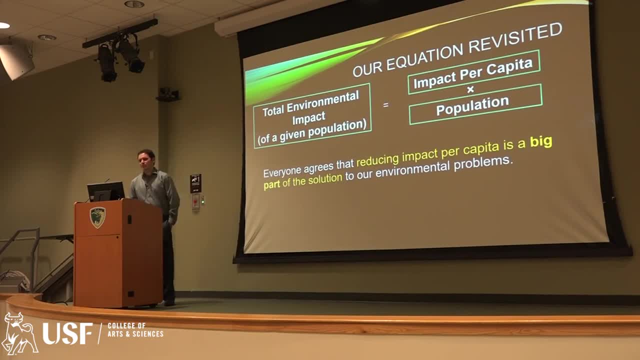 to solve these problems long term. But the issue that we run into with this stuff is that the problems are are so wide-reaching, so entrenched and so difficult. maybe we have to do more than just that, Because progress on reducing impact per capita. 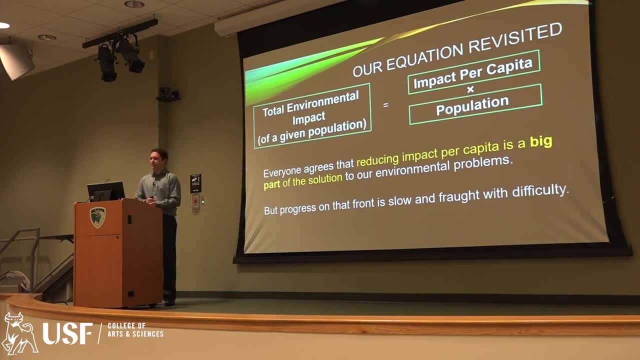 is very slow and often fraught with difficulty. Frankly, people don't tend to want to give up their carbon-intensive lifestyles for a variety of different reasons. What's interesting about the population issue is that there are conditions we can create where societies will voluntarily choose. 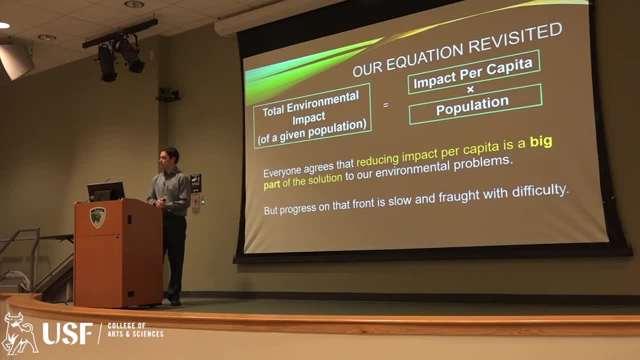 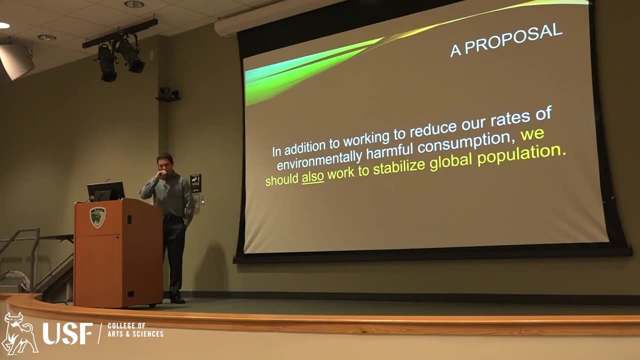 to have smaller families and where societies will voluntarily choose to have fewer children and to shrink their population size. So here's kind of the main proposal. In addition to working to try to reduce our rates of environmentally harmful consumption, we should also try to do something. 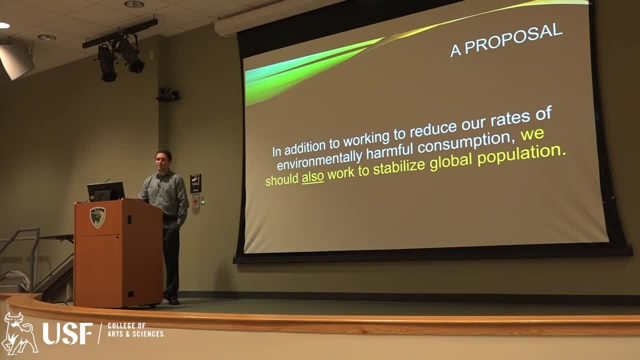 to stabilize population growth sooner rather than later, and in regions where it's possible, maybe even reduce local populations. Now, as soon as a lot of people are on board up to this point, they recognize the contribution that human numbers make to this. 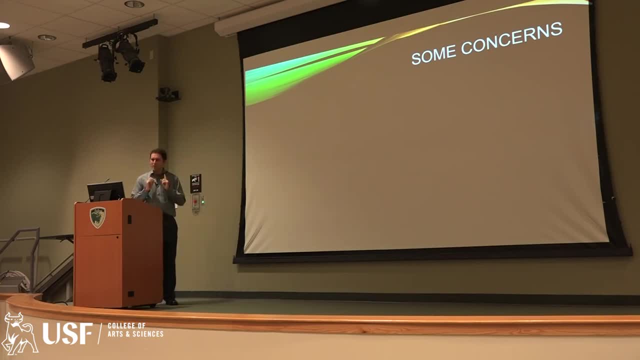 they get it, But when we actually talk about doing something about it, that's where people get hesitant, And the main reason is because there is a history with population policy that is not so great. So specifically again, not a complete list of everything- 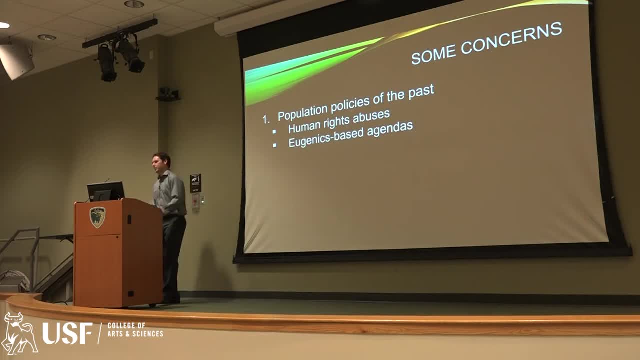 that could be up here, but the two biggest things that people are concerned about is that population policies of the past have often been motivated by eugenics-based agendas. There have been some instances where population policies were specifically designed to, say, prevent the poor from procreating. 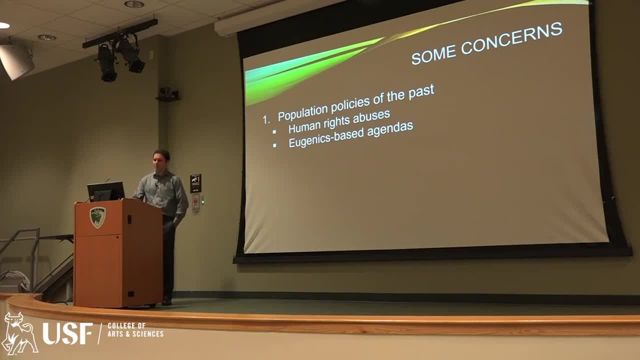 as much as wealthy. There are also instances of various human rights abuses. These are often associated nowadays with China's one-child policy. There are lots of documented cases of forced abortions, forced sterilizations In some of the other policies that were put into place. 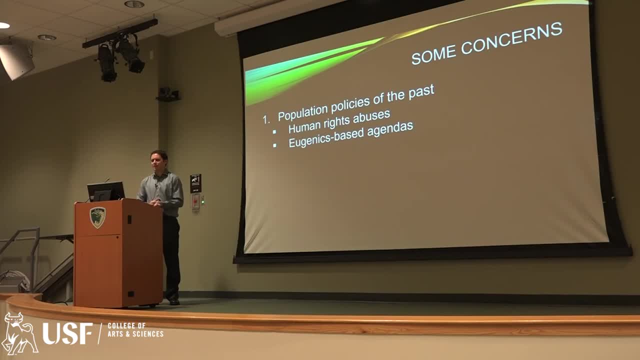 in other countries, like India, there are well-documented cases of getting sterilizations from people without their informed consent. So giving a consent form to someone in poverty who can't read, getting them to sign it, oh great, here we'll sterilize you now. 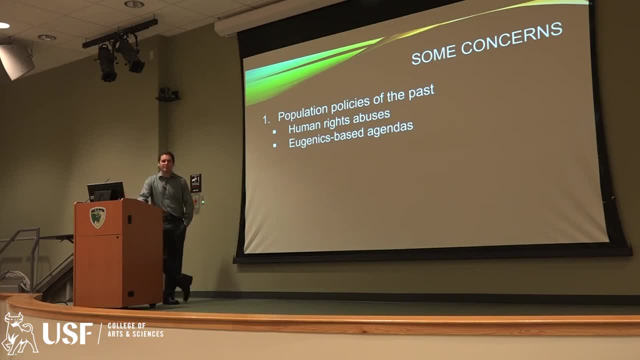 Obviously, these kinds of things are deeply disturbing and things that people do not want to see repeated. So when you start talking about population, this is the kind of stuff that people think you're talking about, and there's a sort of repugnant response to that. 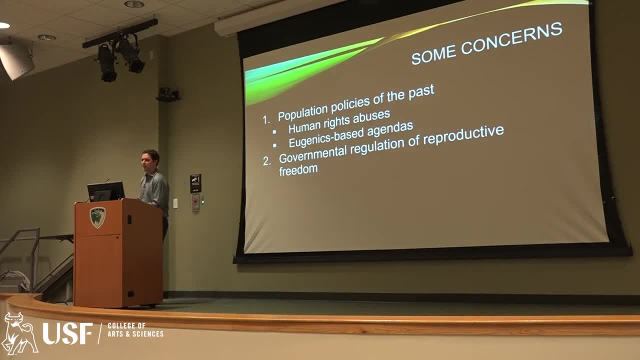 The more general concern that a lot of people have is that the government will now become involved in decisions that they perceive as personal, that the government will actively try to regulate procreation and violate people's rights to reproductive freedom. There is also a gendered component. 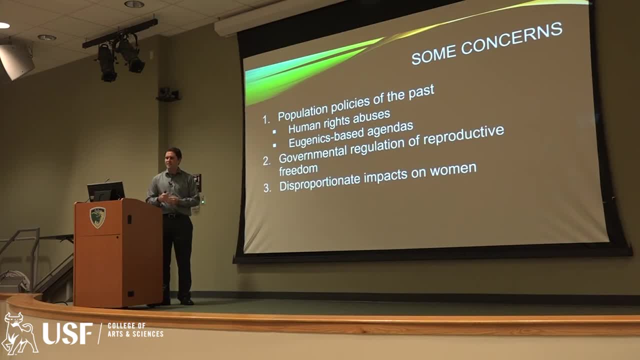 to this issue, because it's not if the government is regulating procreation. if you do have these kinds of violations, it is not the case that men and women are impacted equally. The people who are impacted the most are going to be women, because of the asymmetrical role. 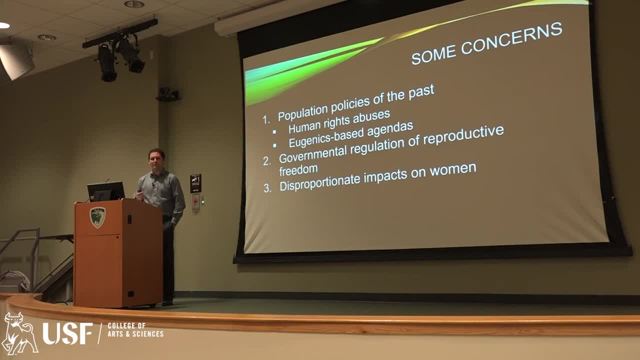 that women play in the process of rearing and raising children, not just biologically, but also socially, in most places around the world, And so if you have some of these other problems that are coming into the play, it's going to also involve gender inequity. 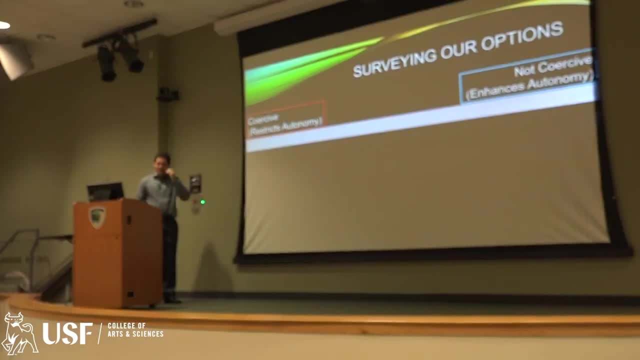 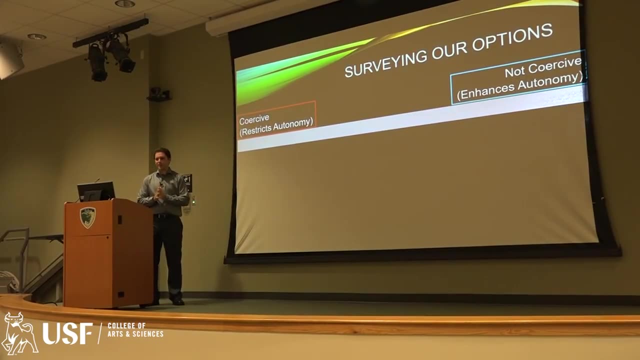 on top of it. But I have some good news, and the good news is we don't have to be talking when we talk about population. we don't have to be talking about really, really stringent one-child policies or things like that. 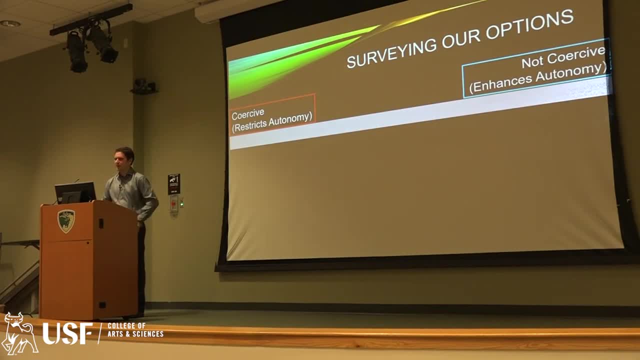 We don't have to be talking about human rights abuses and we don't have to be talking about that kind of government interference. We can talk about population by focusing on the fact that, again, we're focusing on other things. We have a large spectrum of different options. 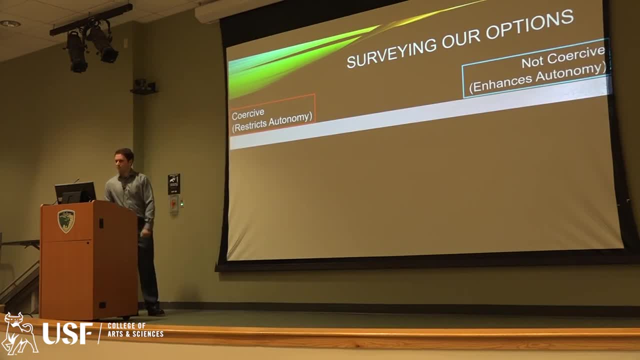 ranging from extremely coercive options that really, really restrict your autonomy, by taking away some of your free choices, say, or by pressuring you heavily into doing something. But we also have options on the other end of the spectrum that are not coercive at all. 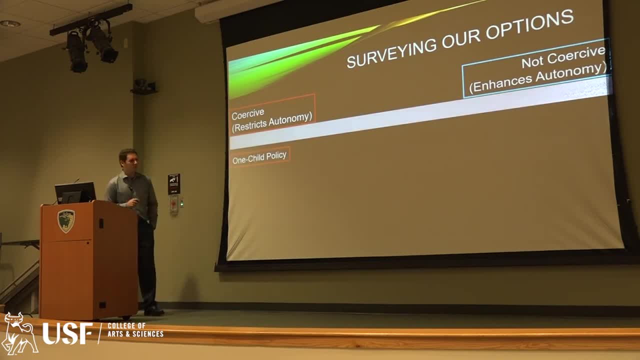 and, in fact, might even be autonomy-enhancing. So the paradigm example of a coercive policy is a one-child policy right, Something like what was in place in China, a policy whereby there are tremendous penalties associated with having more than one child. And if you have an additional child, your second child, for example, wouldn't be able to find a place in a good school or would be essentially like a shadow citizen, wouldn't have full legal rights whatever. But there are also things on the other end of the spectrum. 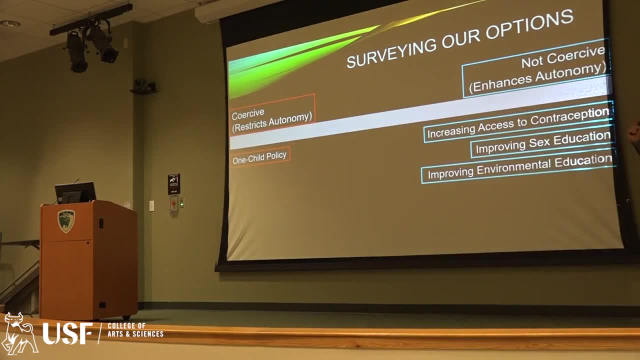 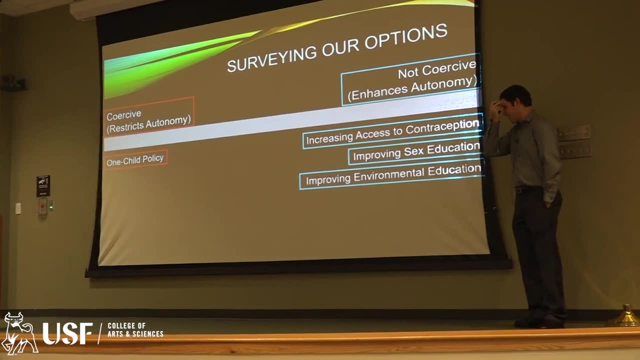 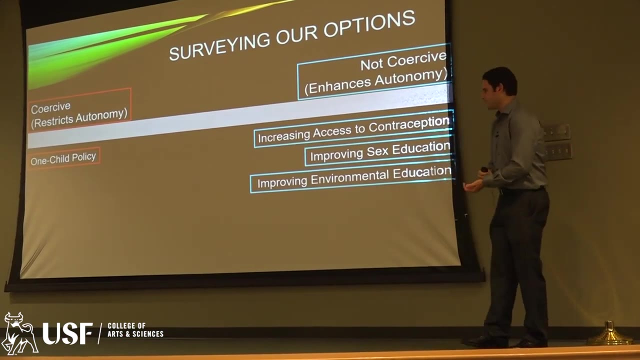 that can be considered that would play a significant role in addressing population. The most obvious one is increasing access to contraception, giving people more access to means of preventing pregnancy. Another one is improving sex education, In other words, for the most part, teaching people how to use those measures effectively. 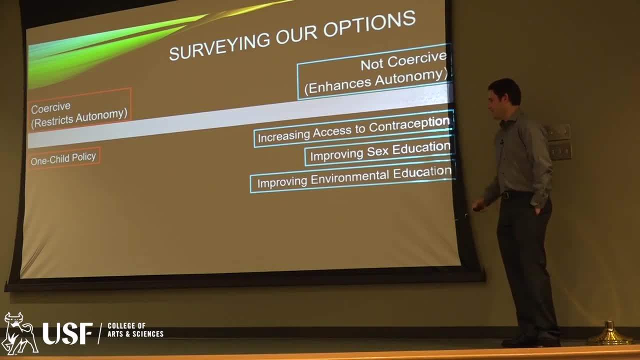 and giving them a sense of what their options are. And the third, which is not as obvious but there's been some interesting recent literature on it, is improving people's environmental education, making them more aware of the impact of procreation and the connection that it has. 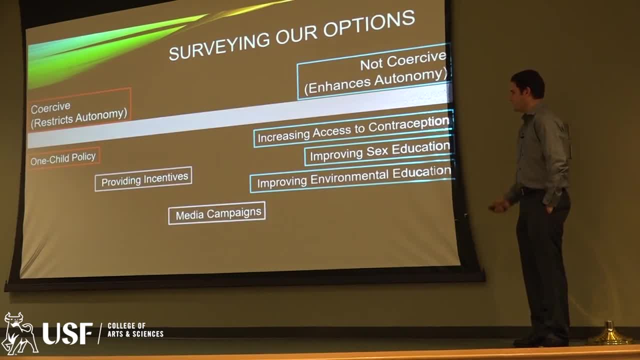 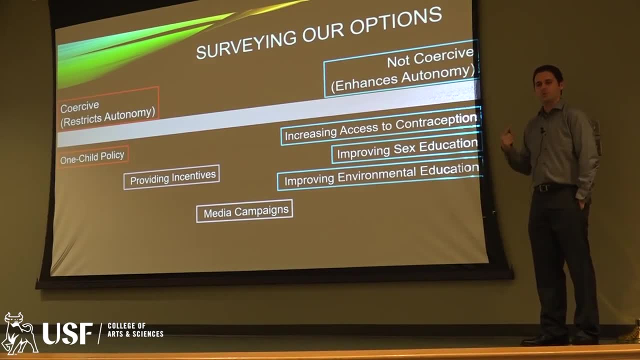 to these other environmental impacts. There are also two that don't neatly fit into either of these categories. You could do media campaigns to promote the idea of having smaller families. In some cases in the past this has been done. for instance, 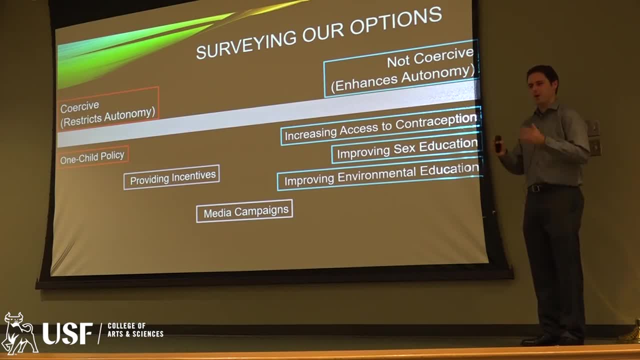 They've been somewhat crude. Singapore basically just put up posters that had two parents- one standing here and one standing here, and then one child in the middle of them. that just said one is enough. They're not winning any points for subtlety on that. 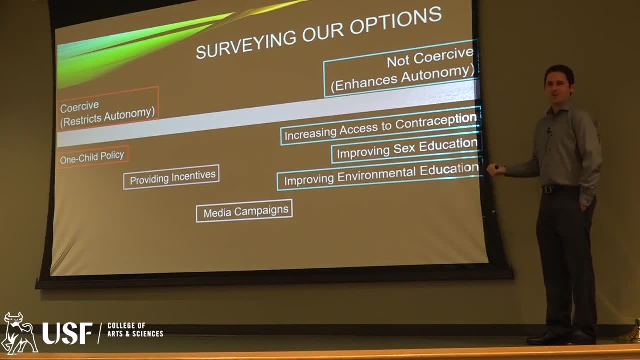 But that's one way, But there are also some that are a little more creative. In a few countries you had telenovelas that were run which, as I understand it, is essentially like the Radio Oklahoma sitcom, And they chose to portray the families in those shows. 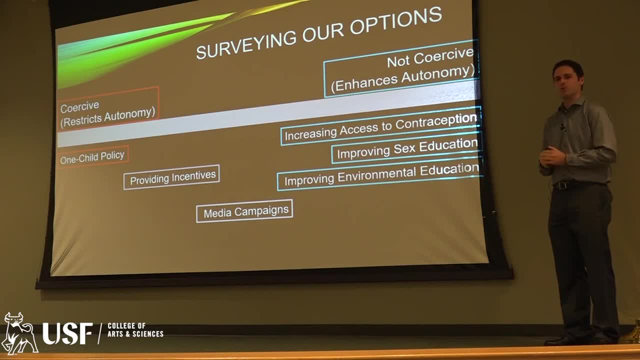 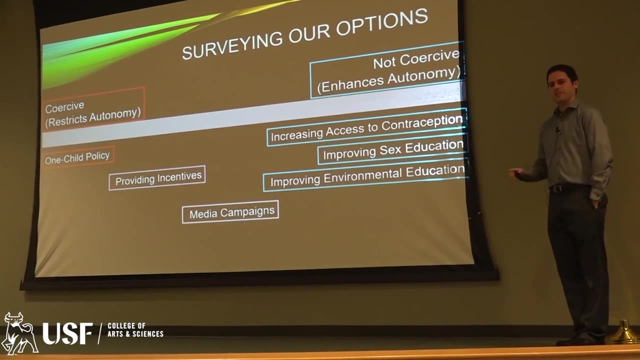 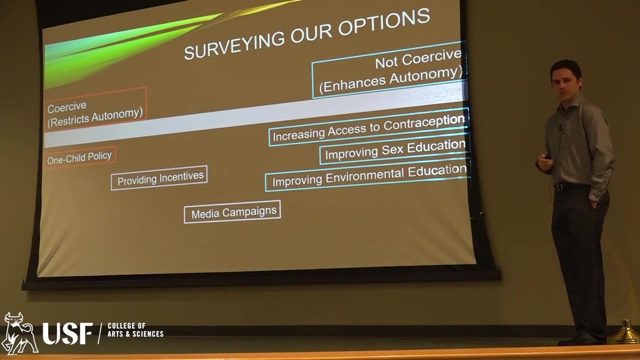 as having smaller, like just one or two children, instead of the Brady Bunch-style family archetype. And what was interesting is when they surveyed people after they had been watching those shows for a while, their attitudes towards small families had changed, had shifted, from when they filled out those same surveys. 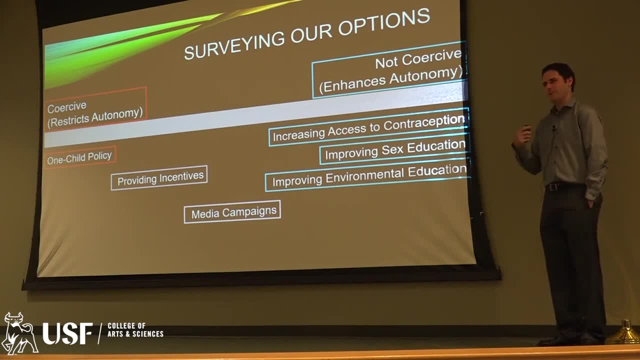 before watching those shows They started to think, eh, maybe having a smaller family is acceptable, could be good, et cetera. Now, a little bit further over, closer to the coercive side probably than the autonomy-enhancing side. 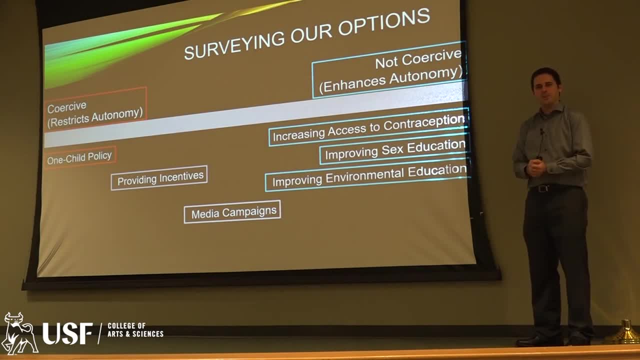 is providing incentives. So providing incentives in extreme cases would mean punishments for people who violate certain agreed-upon standards. That's where we get into territory very, very close to a one-child policy or something like that, Because if you don't have a one-child policy on the books, but if you're saying: well, hey, once you're a second kid, we're going to fine you $25,000, that's effectively in practice going to function the same way as a more stringent one-child policy, But you can also have incentives. that go the other way, that are more positive, Like, maybe you qualify for certain financial benefits by virtue of having a smaller family, Or maybe you provide, as an even cruder example, cash incentives for people who don't want children to be under seconds. 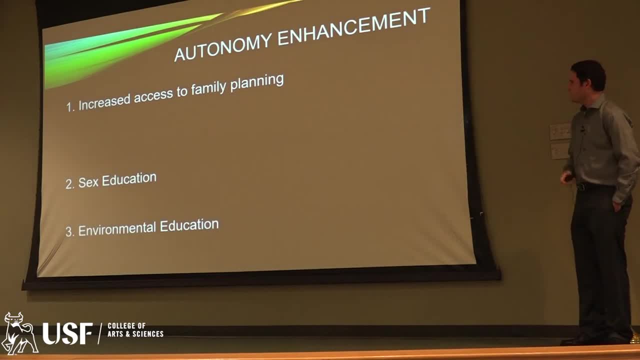 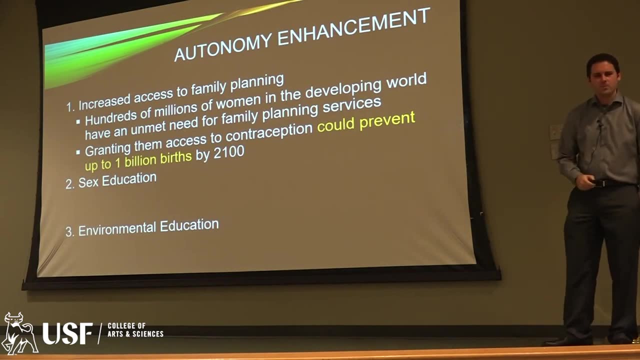 or something like that. So let's look a little bit deeper at the autonomy-enhancing options and think about what differences could make. The one issue on this list that everybody I've seen who's writing about this, thinking about this, seriously agrees on is 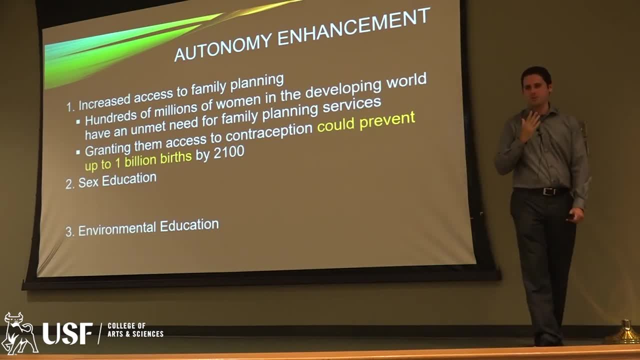 increasing access to family planning services is the big one. This is the closest thing we have in this issue to a no-brainer. There is a huge unmet need for it in various parts of the world. I've seen statistics suggesting that just by providing 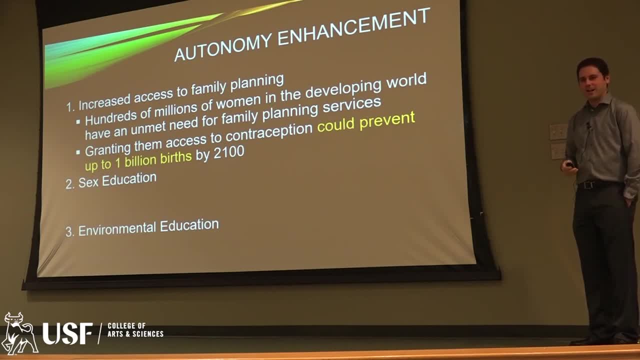 the two to three hundred million women in sub-Saharan Africa with access to contraception who want it, we could prevent up to one billion births by 2100.. If we just give those women the opportunity to have the family size that they wanted and the freedom to make those choices. 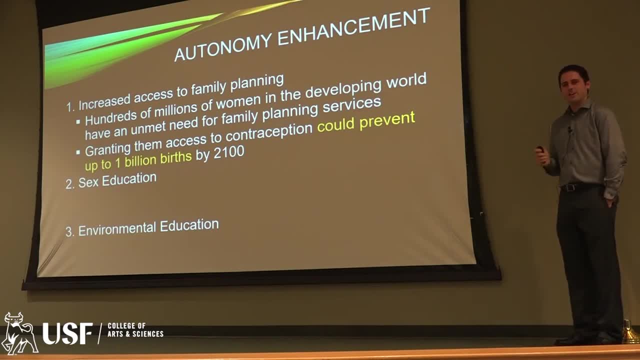 The issue in those contexts is not a matter of coercing people to do the right thing. It's just giving them the ability to make the choices that they already want to make, Just giving them the means to do that. But in some parts of the world, 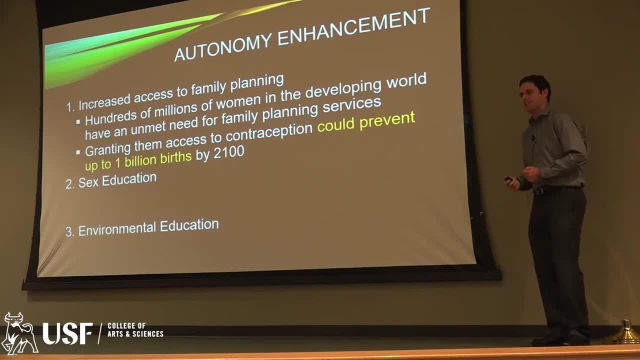 it's not necessarily about increasing access to family planning. It's not an access issue necessarily. Sometimes it's about knowing what to do with that access and understanding the importance of the situation. So around 41% take one or two percent of pregnancies worldwide. 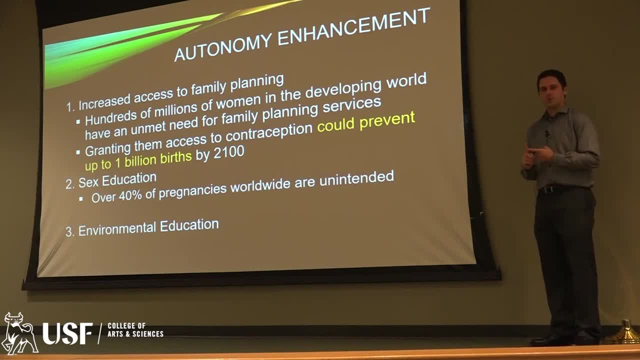 are unintended, which means they were either totally unwanted or they occurred at, in some sense, the wrong time. They occurred at a point in the person's life when they would rather not have that child. That's two out of five pregnancies, which seems like a lot. 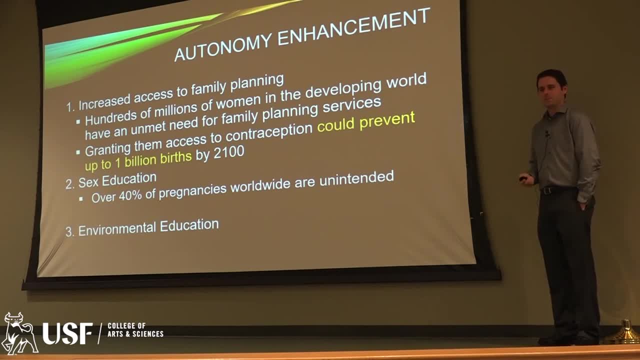 And a significant number of them, perhaps to no surprise, occur in young people, And one of the things that contributes to this is a lack of adequate sex education during teenage years. So in the United States, to use a sort of near home example, 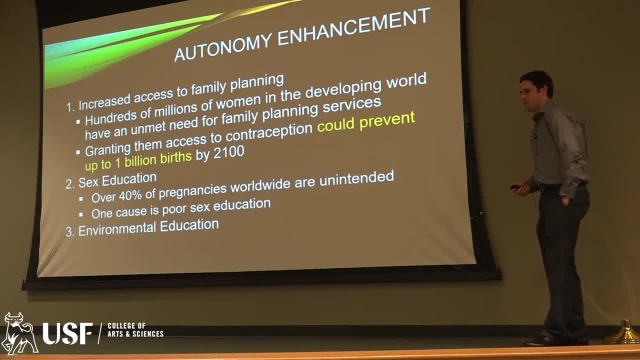 we still have a lot of funding for abstinence-only education, which is an incomplete program, And the data on abstinence-only education is not favorable. There are some studies where, looking at rates of STD contraction- the age at which people self-report losing their virginity- 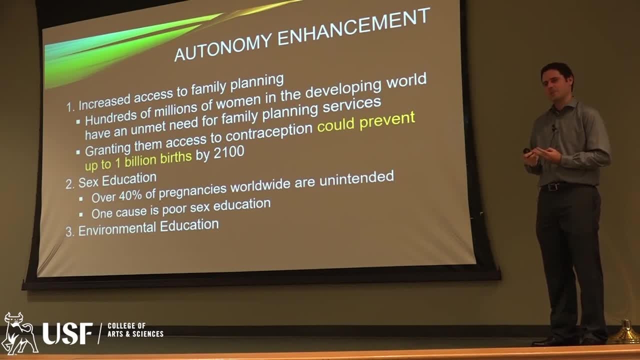 and the rates of teen pregnancy. abstinence-only sex education literally does worse than no sex education, Because if you don't have any sex education you might go on the internet, and there's a lot of information on the internet. Some of it's wrong. 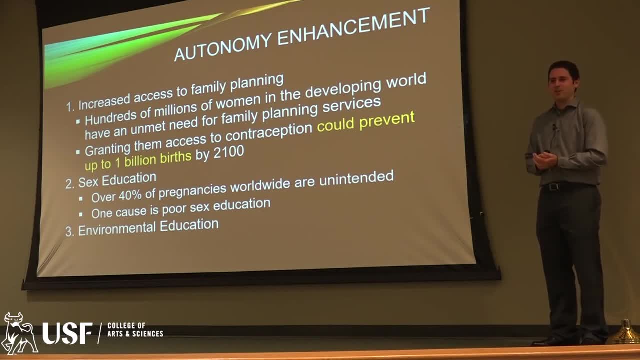 but some of it may also be accurate, And so if you're not getting that information from any other source, you know kids these days will use Google. they will find things. Some of that information will be kind of accurate, But the best information that people get. 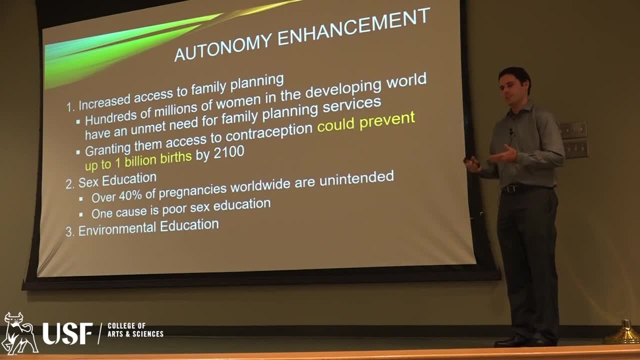 is through comprehensive sex education, which explicitly teaches them about sexually transmitted infections, how to use various types of contraception, most notable being condoms, and how to seek out family planning services that are available to them. Having access to that information is really important if we want these people. 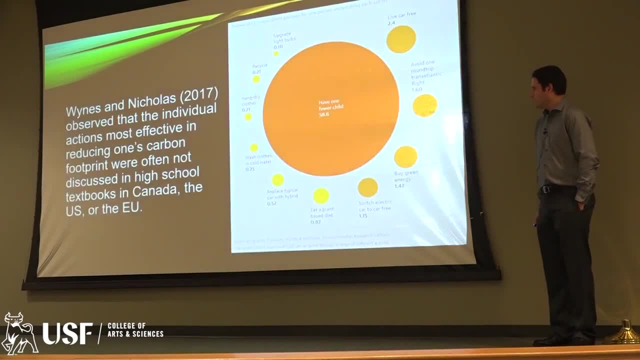 to be able to make informed choices. The other one at the bottom here, environmental education, is not as obvious. The biggest contribution I've seen recently on this was a publication of environmental research letters by two fellows named Wines and Nicholas, And what they did was. 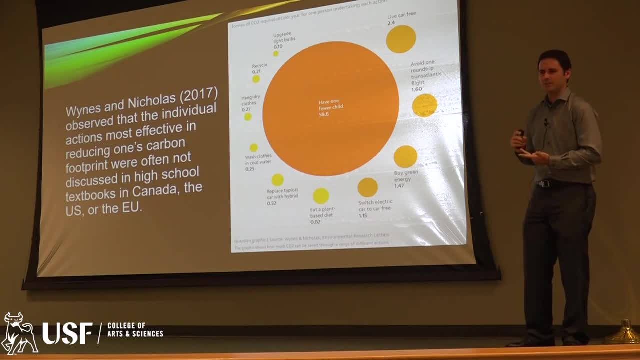 they went through a bunch of high school textbooks in Canada, Europe and the United States And what they discovered was most of the individual actions that were emphasized in trying to help people live a greener lifestyle, so to speak, or lower their individual impact. 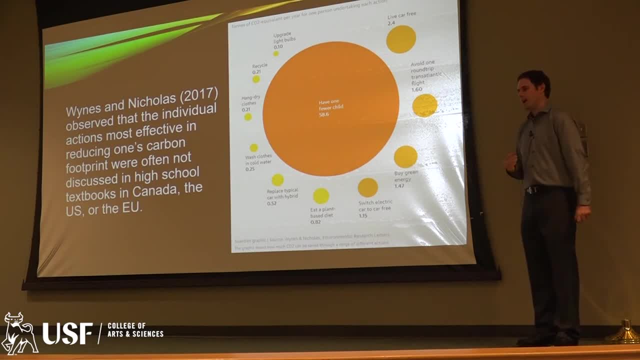 on the environment. most of the actions that were mentioned were not particularly effective. So two of the things this graph is designed to be. some of you, especially in the back, won't be able to read everything, I imagine, but this is designed to be. 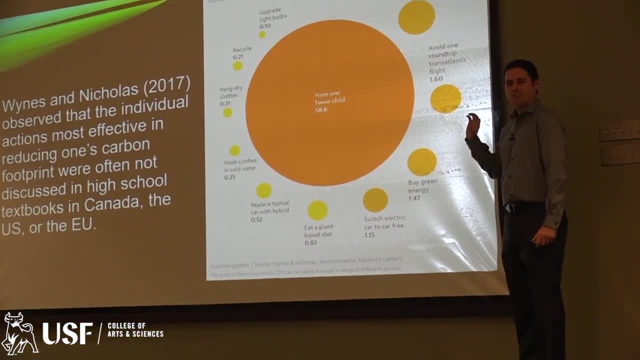 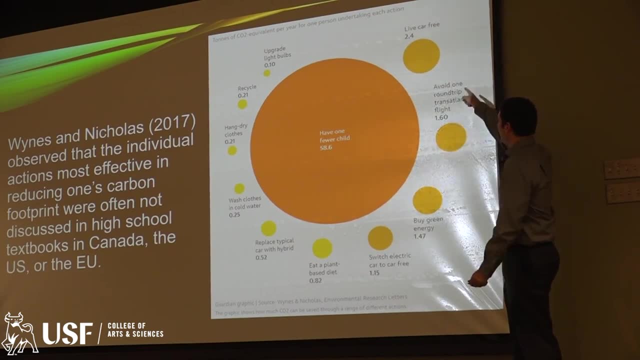 a representation of various actions that you could take to try to reduce your individual impact on the environment And the measurements here. so this says 1.6,, this says 2.4,. these measurements are in terms of your carbon footprint. So if you were to refrain, 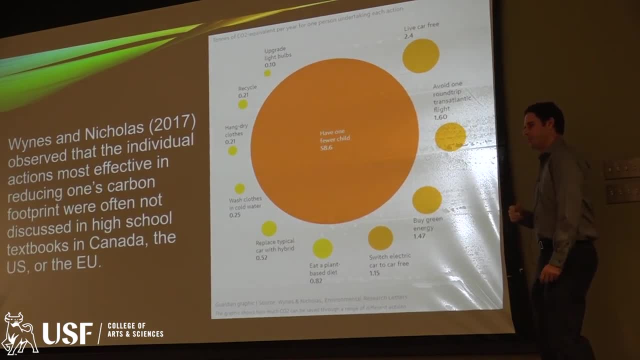 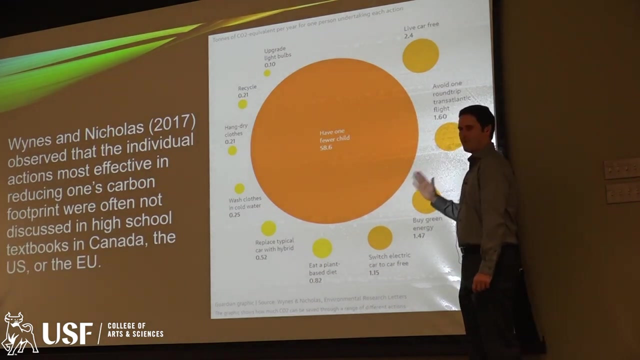 from taking one transatlantic flight. you would save that particular here 1.6 tons of CO2, equivalent relative to if you took that flight. Some of the measures that often show up in these textbooks are things like using the crazy twisty spiral light bulbs. 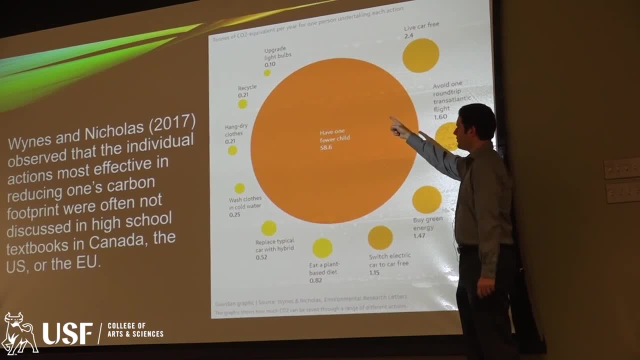 that are more energy efficient, But that only saves you 0.1 tons of CO2 equivalent annually, even if you switch out all the light bulbs on your own. Another one is recycling, but that only gets you 0.2.. Remember one transatlantic flight. 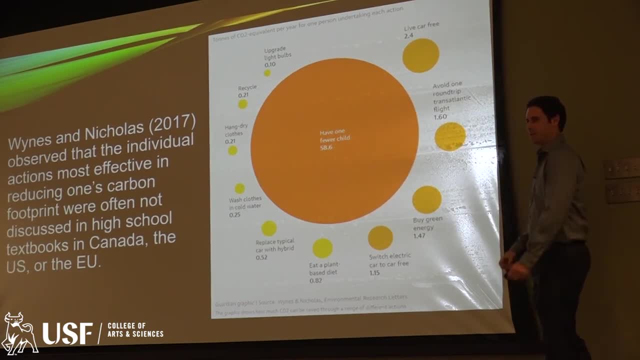 1.6, that's eight times more effective than recycling. if we're focusing on carbon footprint, The one in the center here is having one fewer child, which saves you 58.6 tons of CO2 equivalent. That figure comes from a study by Murtaugh and Slack. 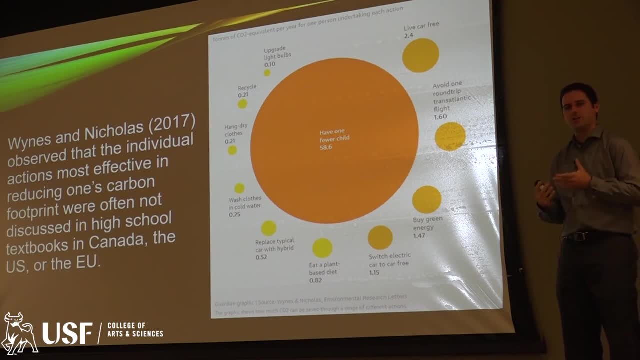 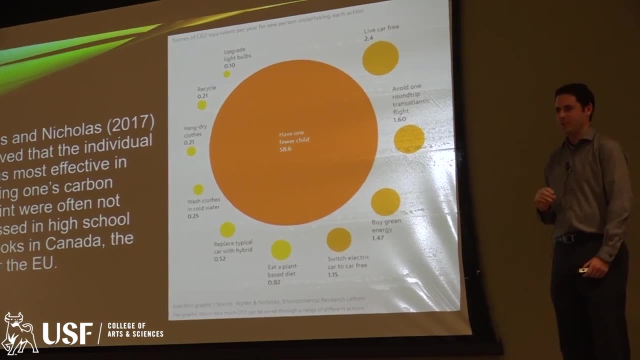 from the University of Oregon back in 2009,, where they calculated the greenhouse gas emissions of your descendants based on kind of a formula designed to track your genetic lineage. So you're responsible for one half of the emissions of your children. one quarter of the emissions. 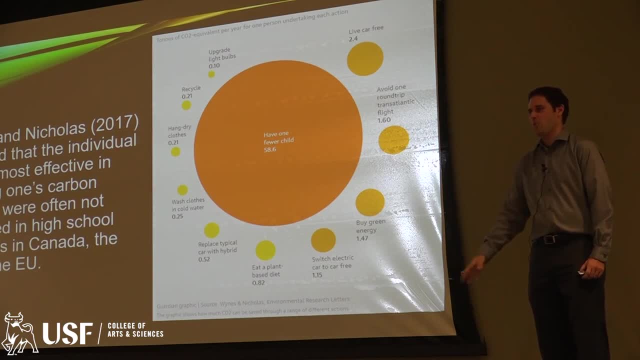 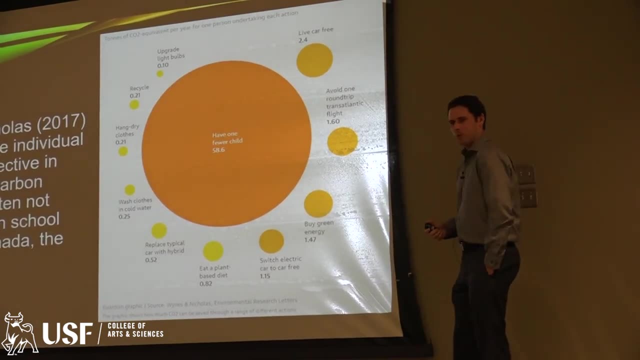 of your grandchildren, because your grandchildren have a quarter of your genes, one eighth of your great grandchildren, and so on. And using that calculation, at least if you live in the developed world, where we have really carbon-intensive lifestyles, having an additional child. 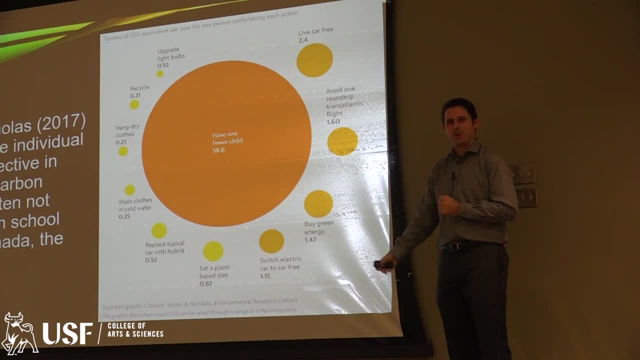 because they are likely to procreate themselves, can very quickly result in a massive increase in your individual carbon footprint, if you understand it that way. There are some controversial assumptions in the background of that study, but I would emphasize that even if you shrink this number down to one tenth, 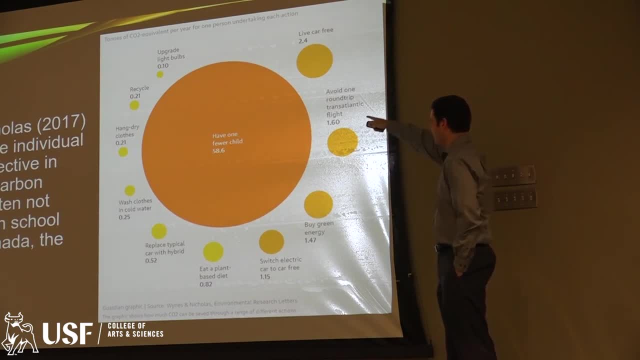 of what it currently is, it would still be by far the most effective action on this list in terms of its annual savings with respect to carbon footprint. But these items: living car-free, avoiding a transatlantic flight, having fewer child, buying green energy. 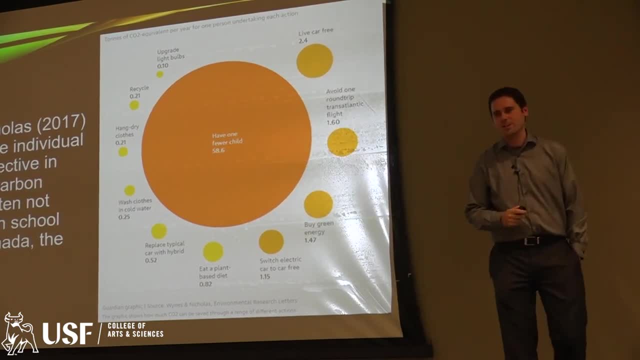 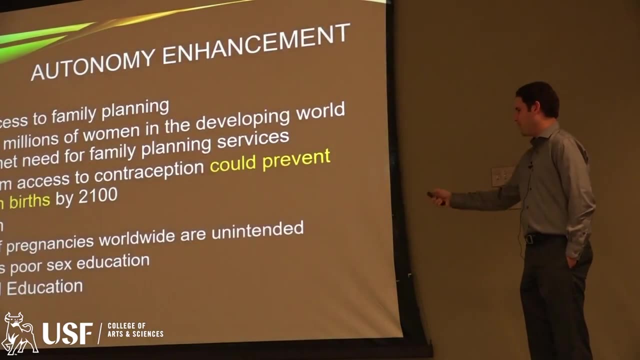 those things don't show up in textbooks in high school. These are not the ones they survey. The stuff that gets emphasized are these more low-impact activities. So, again, one of the things you can do is give people more accurate information. 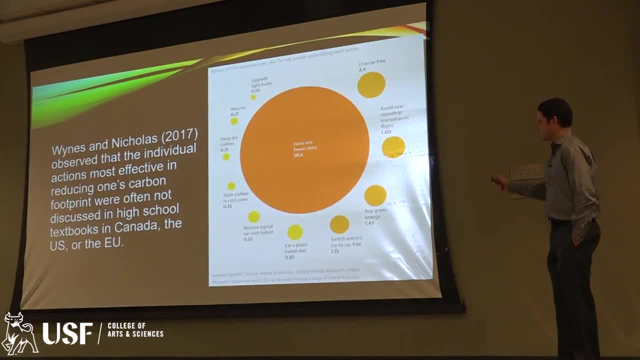 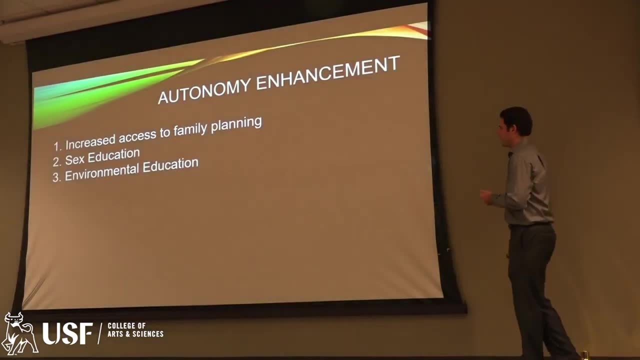 People who care about the environment in the presence of more accurate information may make different choices voluntarily if they have that information. So you notice the theme here. I mentioned that all of these activities are autonomy-enhancing. I want to spell out clearly what I mean by that. 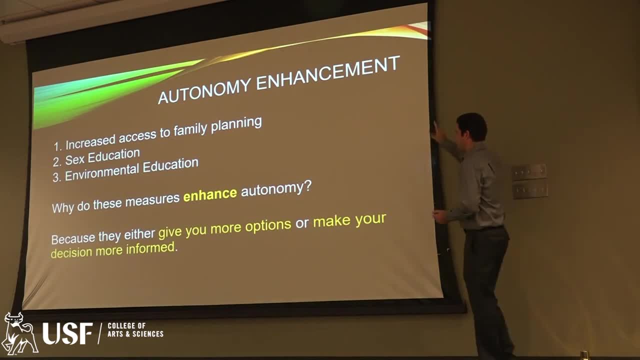 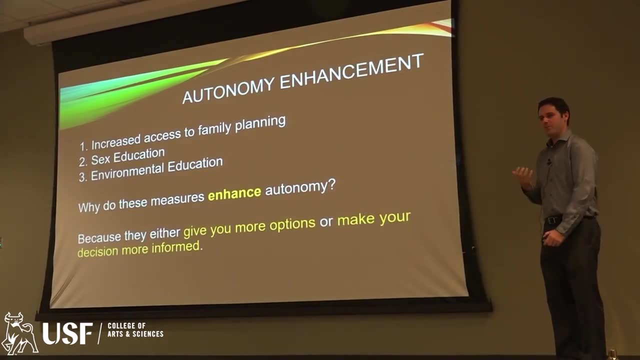 There's no confusion. Increased access to family planning gives you more options, more choices. It gives you more control over how you live your life. That doesn't mean you have to use the options that are available, but it gives those options too. 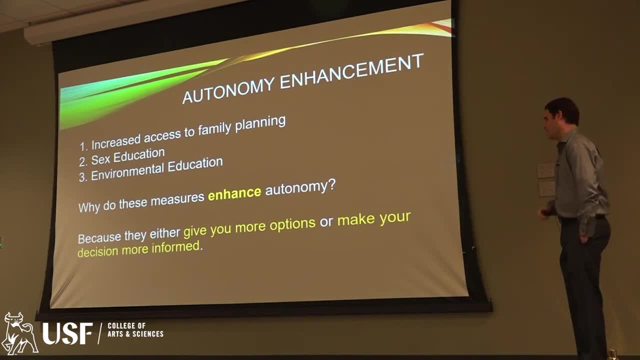 That's why I consider that autonomy-enhancing. The other options increase your autonomy because they make your decisions more informed. They give you more accurate and more complete information, And so because of that, instead of making kind of a halfway-informed decision, 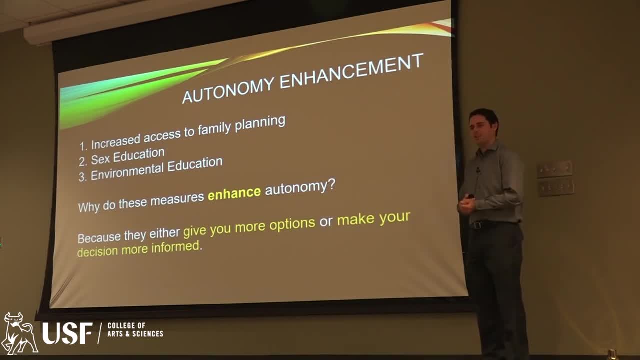 you're actually making a decision that's pretty well-informed. And what about those two intermediary measures? I think there's a lot to be said about those. I think there's a lot to be said about those. I think there's a lot. 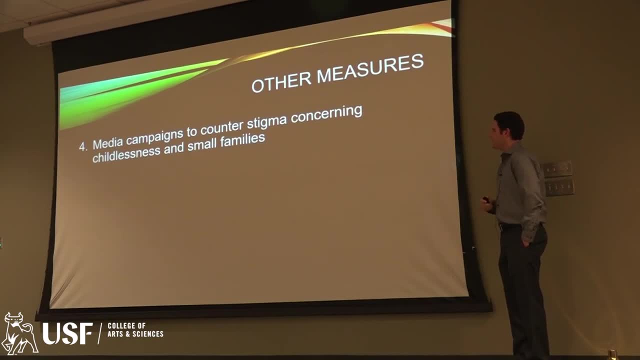 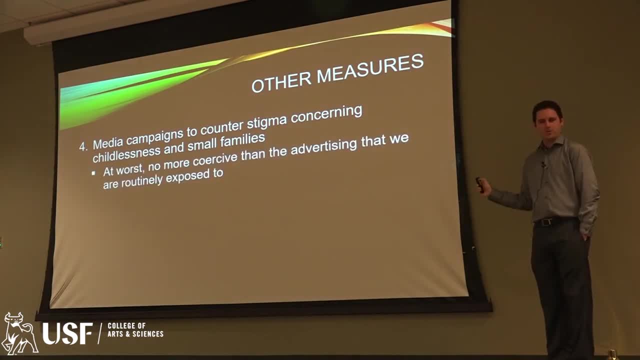 autonomy-enhancing in a kind of interesting way. Now I wanna point out: even if you aren't a huge fan of media campaigns, they're not going to be any worse than the bombardment of advertisements that you see on a daily basis already. Now you may find 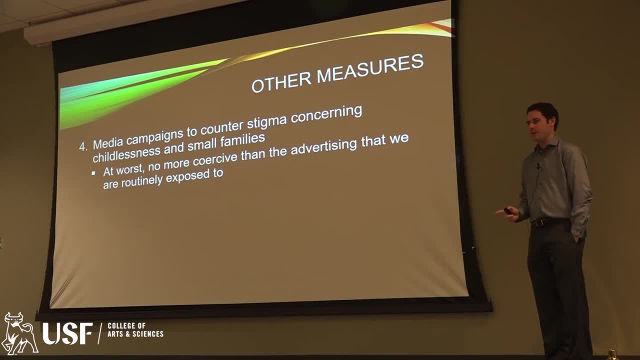 those annoying and tedious- and my god, I don't know how many political advertisements I've gotten in the mail this year- but very few people think that those advertisements are just in themselves unethical. There are some advertisements that can be unethical because they involve, you know, reinforcing say. 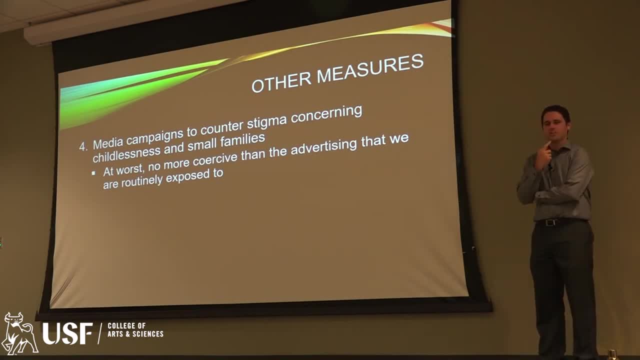 sexist norms or stereotypes or drawing those kinds of things. but most people don't think that advertisements in and of themselves are morally objectionable. So even if they're annoying, even if they're tedious, even if you think of media campaigns, it really just boils down to advertising. I'm not sure if I'm a fan of that Being annoyed. 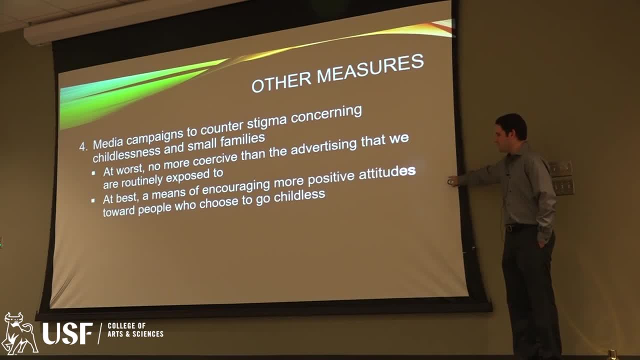 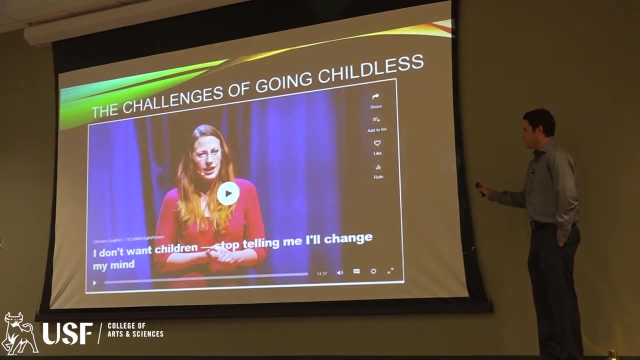 at something is not the same as saying something's wrong. But at best I think media campaigns could be autonomy-enhancing because they make certain kinds of lifestyles more acceptable than they otherwise would be. So I'm not going to like play this talk. This is just kind. 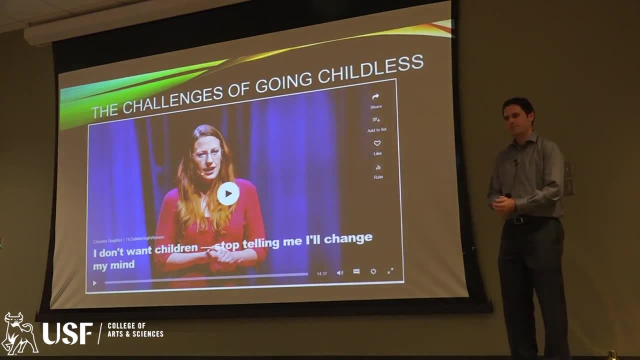 of one resource to consult to get this perspective. This is- I can't remember her last name- Kristen Reiter or Reiter. She has a TED talk that recently came out where she basically recalls her experiences trying to find someone, a doctor, who is willing to let her get a surgical procedure such that 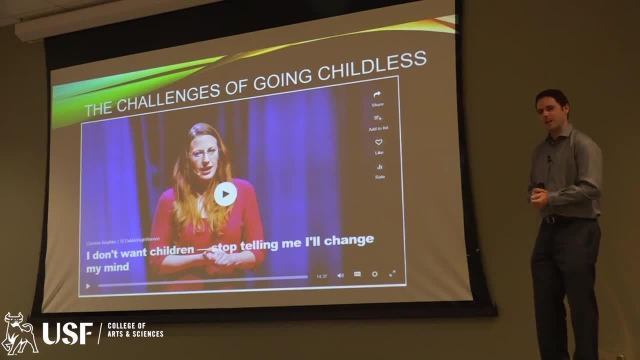 she can't get pregnant again, And it is interesting how hard it was for her to get that procedure, because she was routinely told by medical professionals that she would change her mind about not wanting kids, that she was too young to understand the gravity of the decision. 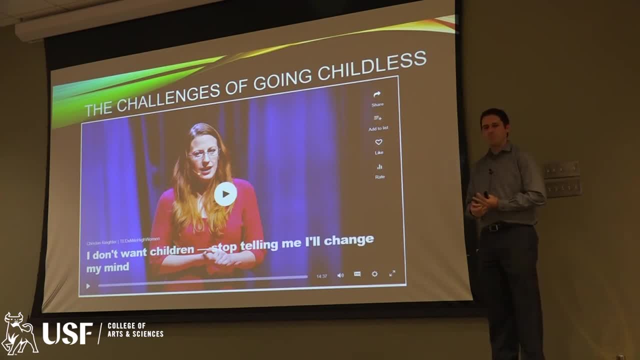 that she was making, that she was not being considerate of her partner's needs, even though her at that time boyfriend was totally fine with it- And in various ways they were very demeaning to her. you know, attempts to exercise her reproductive autonomy And 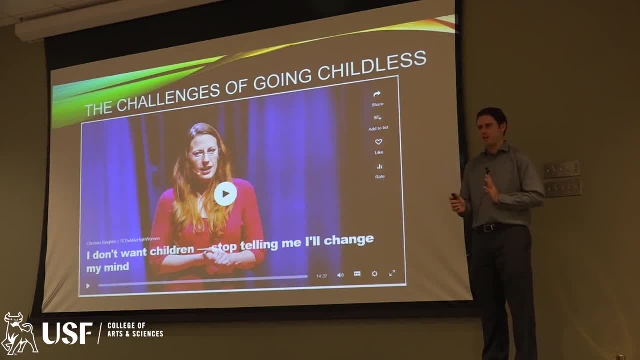 at the backdrop of this, there were probably, in some of these contexts, a gender component to this, the fact that she was a young woman interacting with male doctors who believed that they knew her situation better than her. But a lot of it is also a pro-natalist. 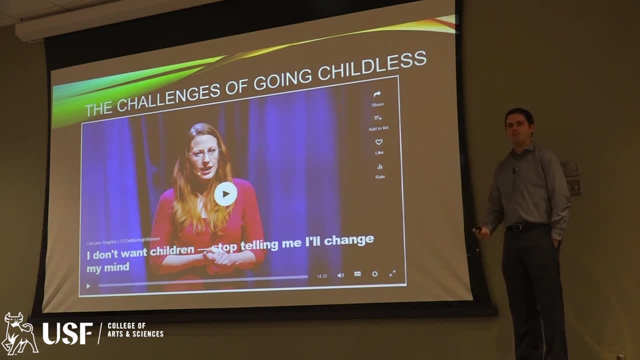 bias in society. So think about how we behave in the context of people who have children. right, We congratulate people on having children, on being pregnant. We don't do that for people who decide to stay childless, Like if someone comes up to you and is like like hey man. 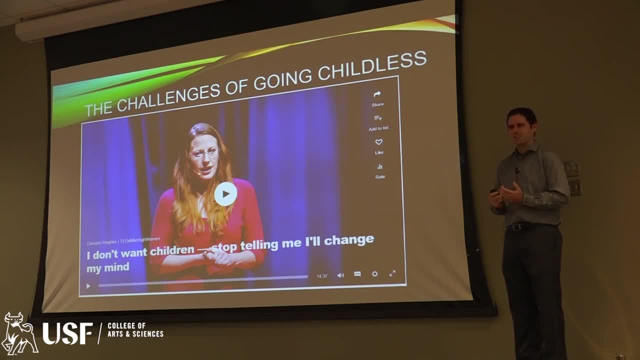 you and your wife ever been having a child And they say, nah, we decided against it. Usually the response will not be: oh congratulations, man, You need to sleep in all you want. It's not usually how that conversation goes. Now I'm. 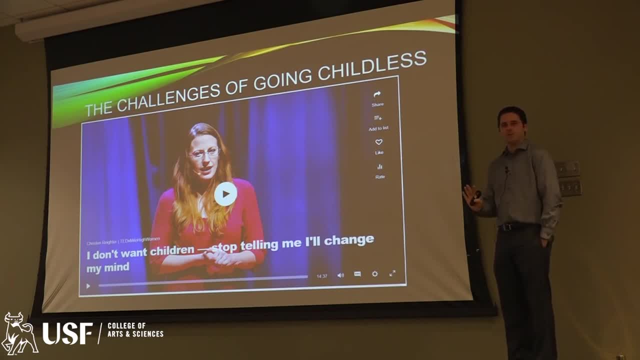 not saying that it's. I'm not in any way saying here that it's inappropriate to you know, celebrate the birth of your child or anything like that. I'm simply pointing out that there's an asymmetry here, that one type of activity, one type of lifestyle, namely raising a family, 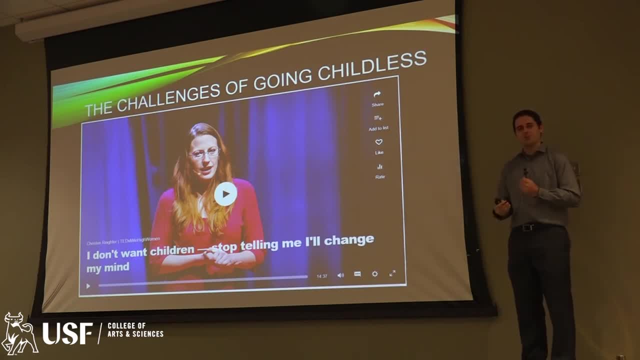 is commonly praised, whereas a decision to remain childless is not, And as a result, there's sort of this background assumption that the normal thing to do, the natural thing to do, the desirable thing to do, is to have a family, And so long as that. 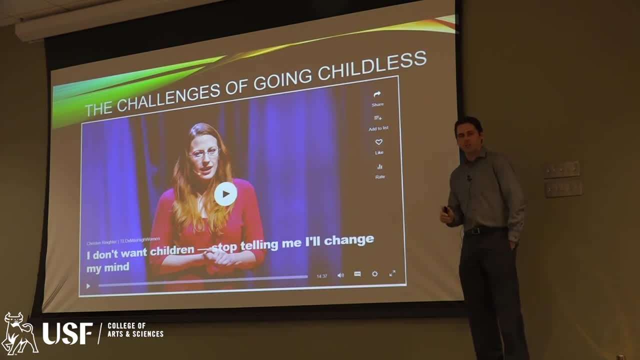 value persists. there are many people who don't really want to have children, who will in various ways be pressured into it or feel like their autonomy is compromised Here. in her case, she was very adamant that she didn't want children. She did not ever change her. 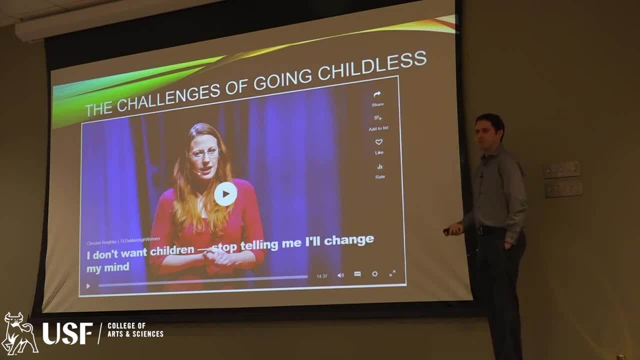 mind on it. She did eventually have the procedure, But it was extremely difficult for her to do. And if we really care about- you know- people's- if the issue here is we really care about people's reproductive autonomy, we should be willing to honor these kinds of requests and to. 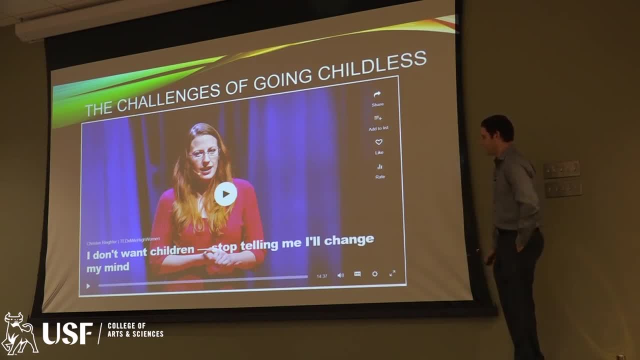 not cry and try to get people to change their minds about this sort of thing. So if media campaigns could help counteract this stigma and help people view a small family, or even the absence of a family with children, as a positive lifestyle, that is acceptable. I think that. 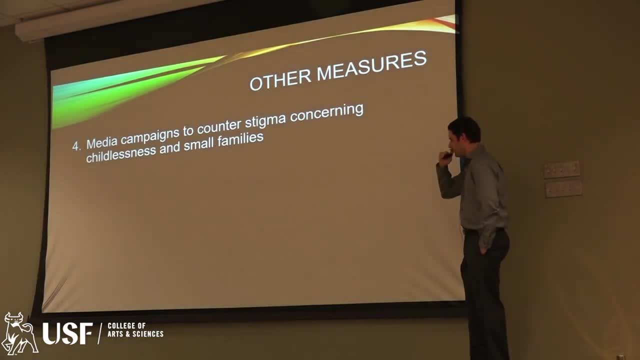 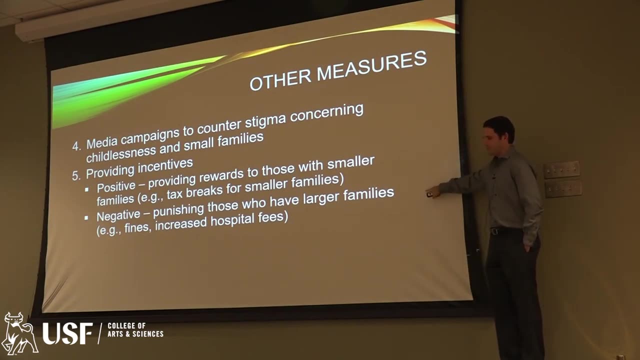 would be autonomy. It would be more enhancing rather than autonomy-restricting. Now I mentioned incentives. already I alluded to these. You can have positive incentives and negative incentives. Negative incentives are like punishment. Positive incentives are more like providing benefits to people. This is where we start to get into murky territory. where we start to go further on the pendulum downstream toward coercion. Really really extreme negative penalties like excessive fines Or increased hospital fees for people who have more than X number of children. That really just starts to look more or less indistinguishable from what a one-child policy or something. like an X child policy. whatever that number is would be, in practice, Positive incentives Harder to assess. I think It's less clear whether those wind up being coercive. You could, for example, provide tax breaks to people who decide to have smaller families. 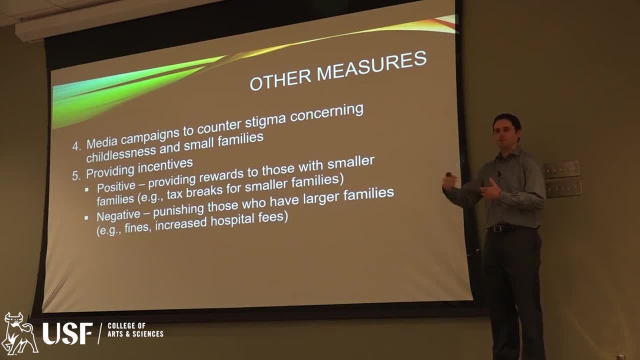 rather than the current system where you provide tax breaks for people, Every dependent you have you get an additional tax break. You could invert that system and make it so you start with, say, four exemptions and every dependent you have, you lose one of your exemptions. or something like that. That would be one way of providing a positive incentive for people to limit their family size in some way. It's not like it would be a punishment. It would simply be a benefit that people who remain children would have, People who remain childless would get, and people who didn't would. Interesting enough. 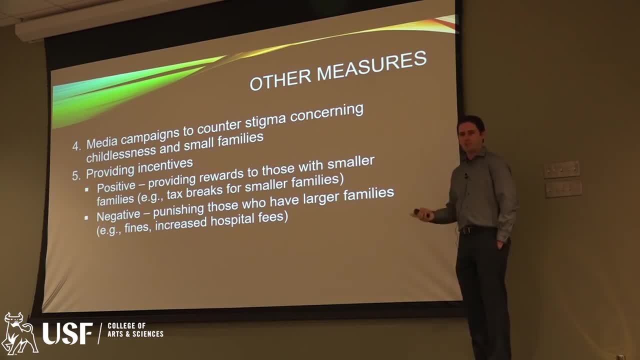 there have been some people who have argued independence of anything having to do with population, that that should already be the system in place, Because if you're childless and you're paying taxes, you're probably paying for things like public school systems that your kids are never going to use. But that's another story for another day. 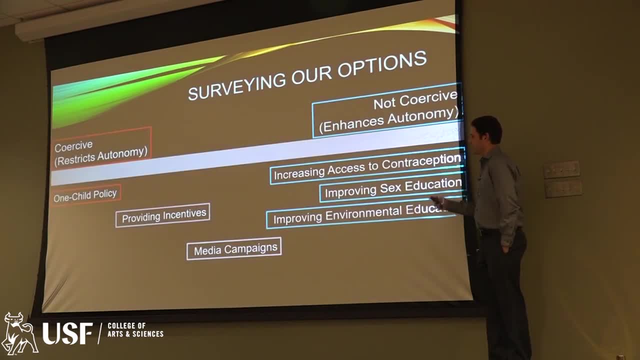 My view on incentives as far as this graph goes, is it's going to depend a lot on the context We're using them, but it would be very challenging to use negative incentives in a way that wasn't coercive. So I think if the goal is to try to stay away from coercive policies and use the tools on this side of the equation, only positive incentives are really going to get much traction: The existence of benefits for people who are childless, but penalizing people who choose to have large families is probably, if the goal again is to avoid, really, really significant. 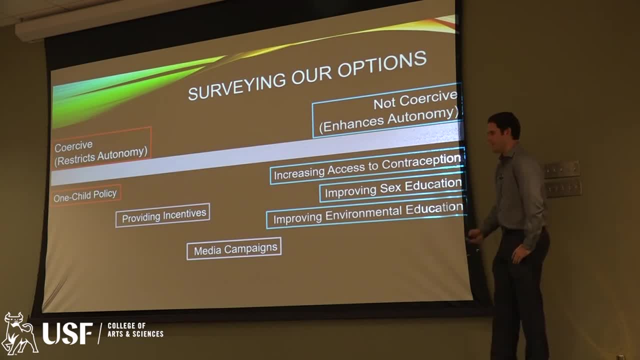 restrictions on autonomy. that's not going to work. You're going to have to stay away from those sorts of things. But here's the takeaway that I think is more important: There's lots of stuff on this side of the board We don't just have to be focused on. 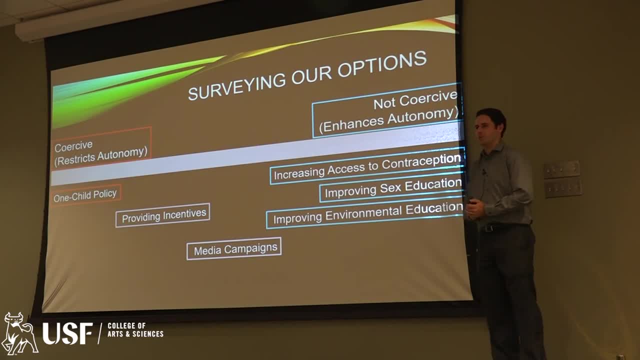 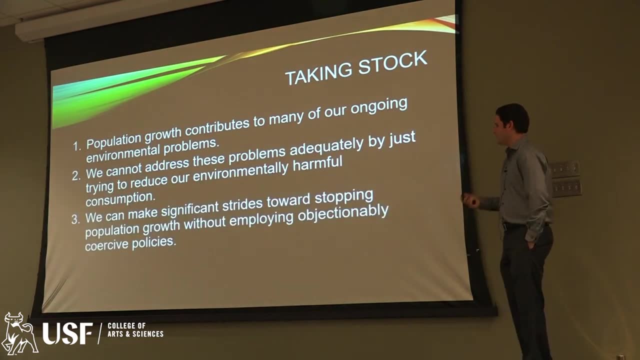 worries about a one-child policy if we want to do something about the population issue. And so what I hope at this point to have kind of convinced you of is basically three claims: First, that population growth is a contributing factor to a lot of our modern problems. 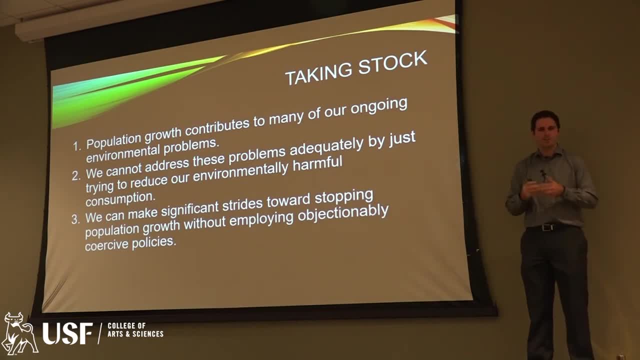 Again, that's not super controversial. Most people can get on board with that and just recognize that it's a factor in play. I've also tried to suggest we can't address these problems adequately, at least if we're trying to do it in the timeframe we have available. 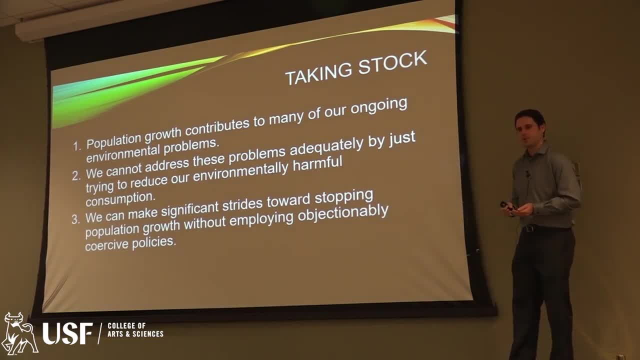 before the problems get really, really bad. This is especially true with climate change. I don't think we can do that by just focusing on environmentally reducing rates of environmental consumption. We have to do more than just that. And third, I think we can make significant 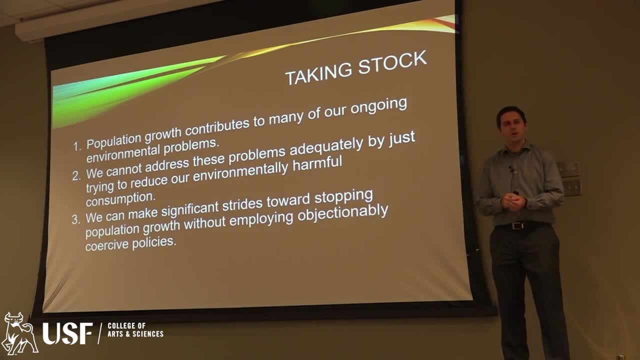 strides toward stabilizing population growth without resorting to extremely coercive measures. We can do this significantly by just enhancing people's autonomy, giving them more information, letting them make the choices they actually want to make, working in various societies to correct a stigma of the environment that is happening to them, and even to working in. 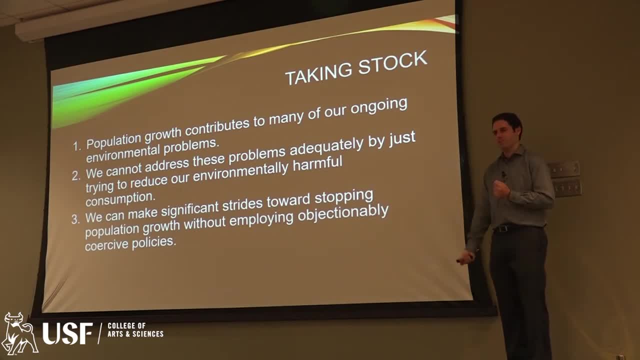 such states where this is actually really important. That's what I think is important. And third, I think we can make significant strides toward stabilizing population growth without resorting to extremely coercive measures. We can do this significantly by just enhancing against childlessness or against small families in general. 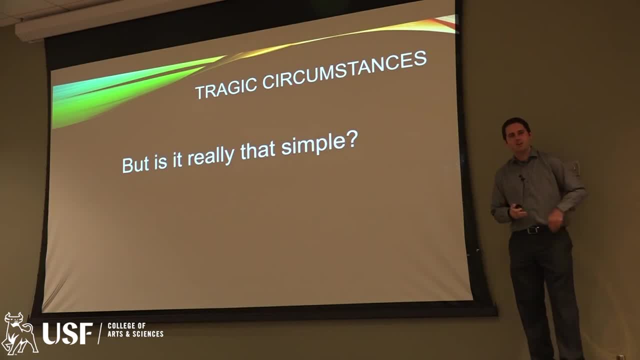 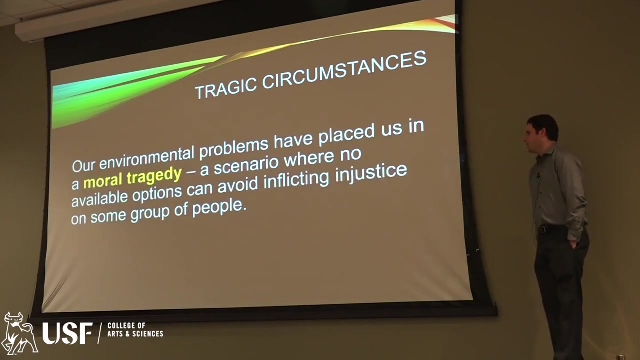 But you might be wondering at this point: is everything really that simple? Is it really that easy? And the short answer is no, because nothing in philosophy is easy and nothing with respect to these issues is easy either. So here's my assessment of kind of the situation. 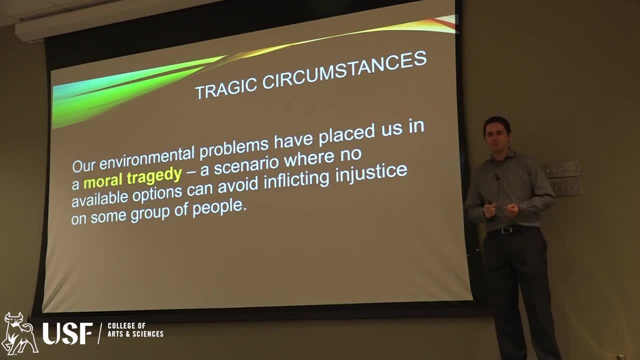 that I compare in. There are some moral problems in the world that admit of easy solutions. So if you are mugged on the street and someone takes your wallet and you file a police report and the suspect is apprehended, your wallet is returned. 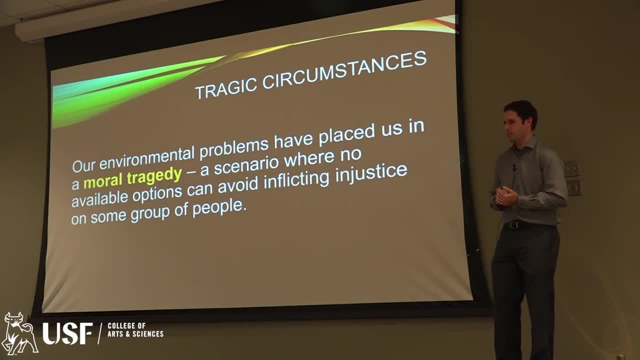 and they're sentenced to 30 days jail time or whatever the appropriate punishment would be in that situation. that strikes me as a moral problem that was satisfactorily resolved. You got back what you lost. the perpetrator was punished So far as a mugging goes. 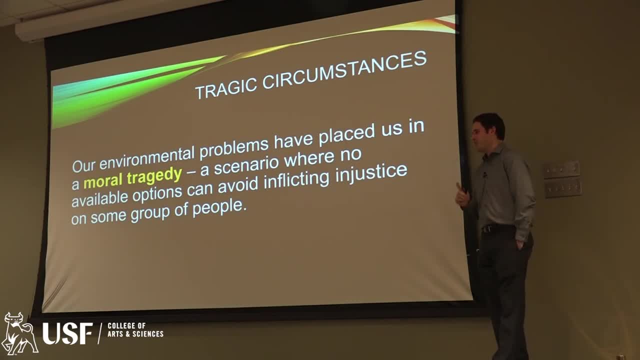 that's a happy ending, right, But very few of our problems at this level of complexity and on a global scale admit of those kinds of resolutions. Sometimes we are in tragic circumstances where there are no easy solutions and where our only choices are between unjust outcome one. 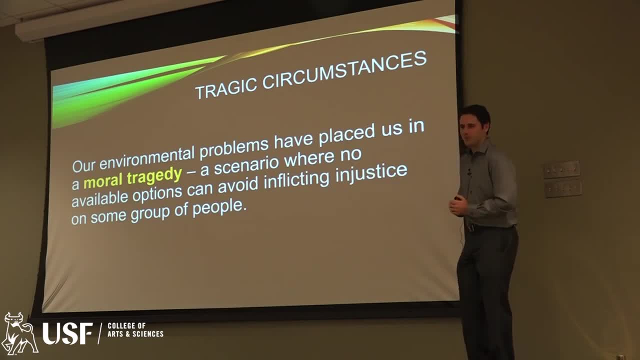 and unjust outcome two or harmful outcome one, harmful outcome two or something like that. So I think that's that's the kind of situation we're in with respect to most of these environmental issues. We are in a situation where loss of some sort, 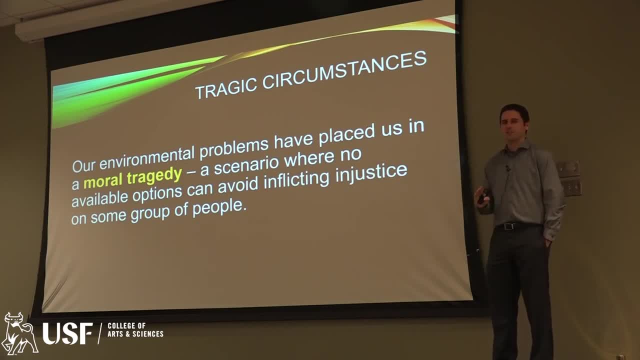 in terms of harm, unfairness, injustice, case violations. whatever is inevitable, It cannot be avoided, And so the question, then, is: how do you deal with these kinds of scenarios when all of your available options involve inflicting injustice on some group of people? when you do. 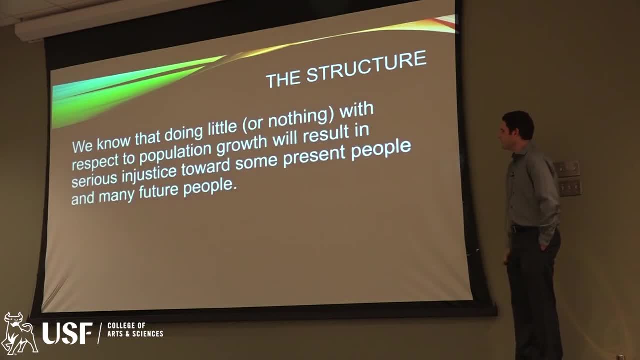 How do you resolve those kinds of things? How do you deal with these kinds of problems? So here's the application to the population issue. We know that doing little or nothing with respect to population growth will result in some injustice for presently existing people and, to some extent, future people. 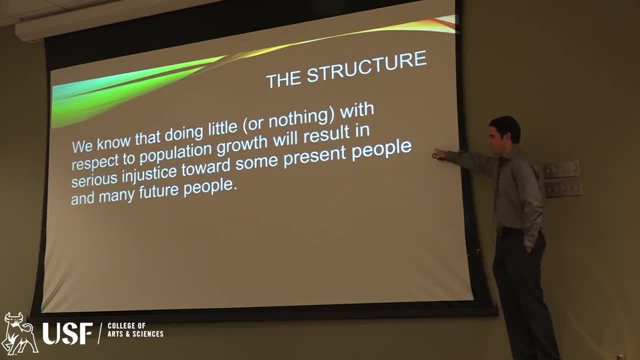 I mean we know a lot more future people will be affected, but the problems are getting so close in terms of temporal proximity that some of us in this room and we'll be affected significantly by the problems that are on that list. So we know doing nothing about it. 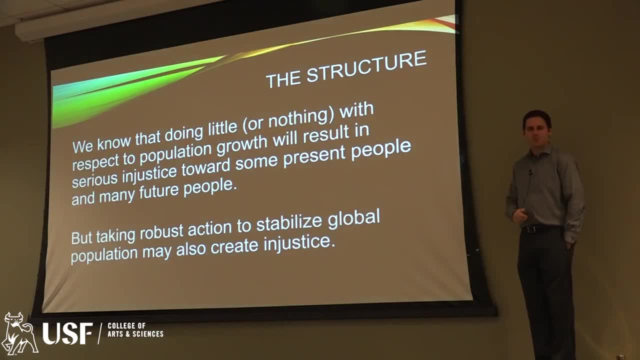 will be a problem. but if we take robust actions to try to do something about population growth, we may inadvertently cause other types of injustice. So it's a sort of damned if you do, damned if you don't type of scenario. So here are just. 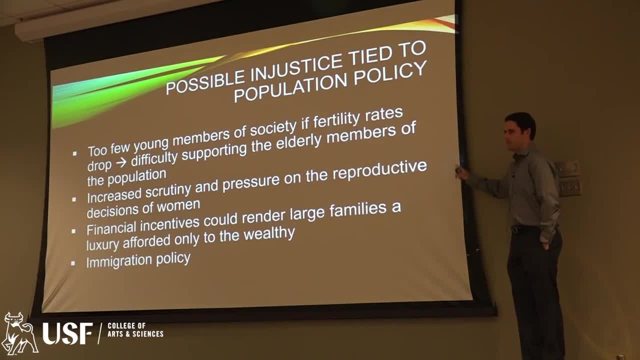 I'm going to go off to these super quick. here are just a few examples of potential injustice outcomes that could happen from trying to pursue population reduction- Really common one that economists will bring up if you have too few young members of a society. 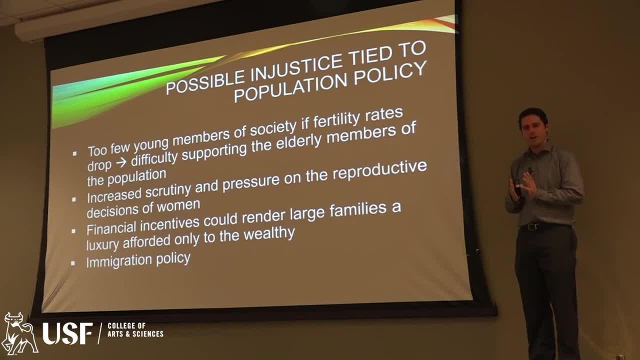 which is what happens when you have fertility rates go way down. eventually you get a much larger elderly population than the working class, and that means it's very, very either the working class has to be really heavily taxed to provide the resources necessary to sustain that elderly population. 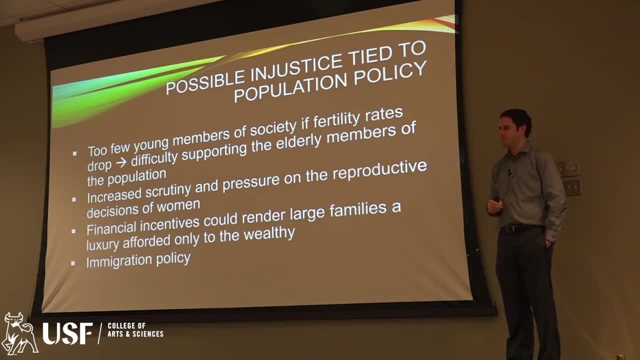 or you've got to make cuts to your medical, to Medicare or other things that provide for those elderly people living life. Either way, somebody's getting the short end of the straw there if you go that direction. This is the kind of scenario actually. 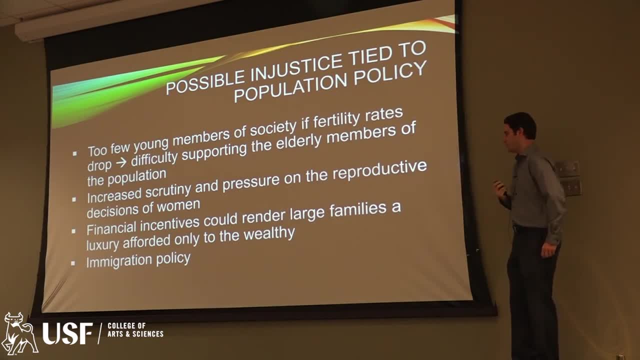 that Japan and Italy are facing right now because they have very, very low fertility rates. You may also see increased scrutiny and pressure on the reproductive decisions of women. Again, like that, gendered asymmetry of reproduction is not just going to go away. 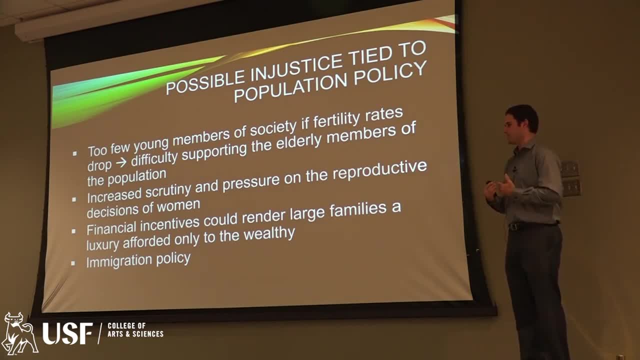 It's going to go away. So, even with the best of intentions, even with creating policies that are as neutral as possible, I think you're still going to see some instances where women are unfairly treated as a result of trying to take populations seriously. 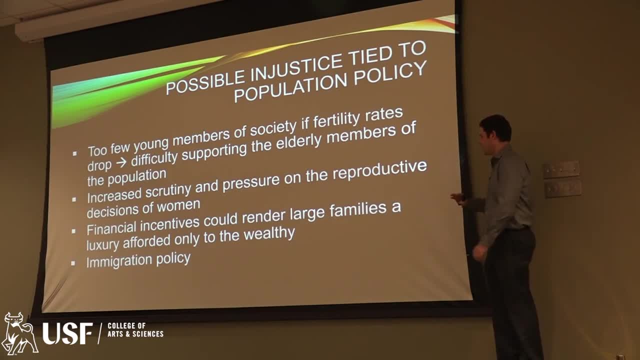 Again, even with the best of intentions, even with trying to do everything in as gender neutral a way as possible, If even positive financial incentives could make large families essentially a luxury of the wealthy, because if you have a pattern of people who are, say, middle class, 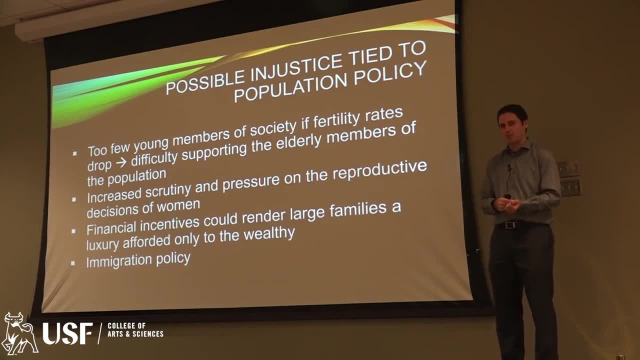 or low-income families recognizing that, hey, I could really use those tax breaks, for example, or whatever other incentives are in play. if they make those decisions persistently, then suddenly there becomes a classist structure of family size where it's only the very wealthy. 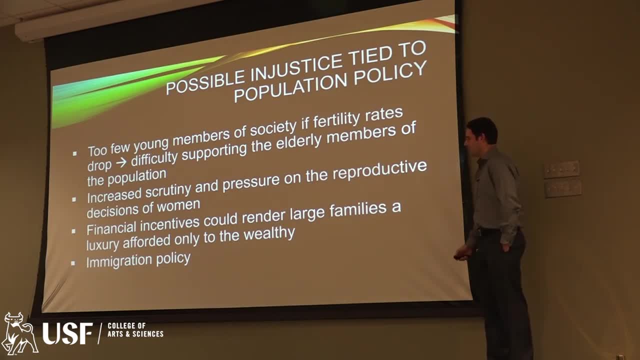 who will end up having large families. And if you are middle class or economically disadvantaged- sort of a foregone conclusion- you won't have a large family. And the last one is immigration policy. Yeah, this is way too complicated to lay out all the details here. But as a quick gloss. basically, in a country like the United States, where our fertility rate is below replacement, our population growth primarily comes from immigration. So if the United States, given its massive per capita environmental impact, wanted to reduce its overall impact, get its, you know. 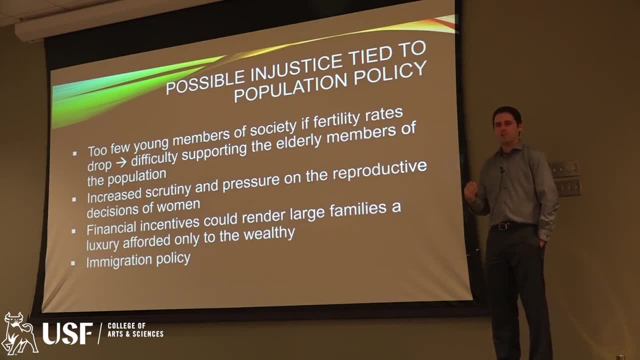 ecological footprint under control. one thing you could try to do would be to halt population growth. You could halt population growth by having extremely strict immigration policy, But doing that may well impose various types of injustice on, say, refugees seeking political asylum to escape terrible circumstances. 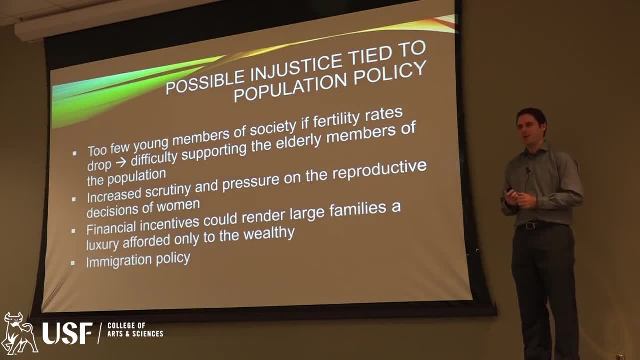 or things like that, And, as a result, you may be in a kind of dilemma where, if there's really there really are no other options for adequately responding to some of these problems, then if you make that decision for the sake of future people, you're screwing over some of the people. 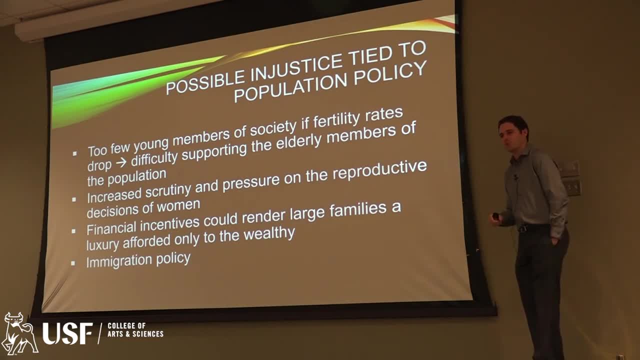 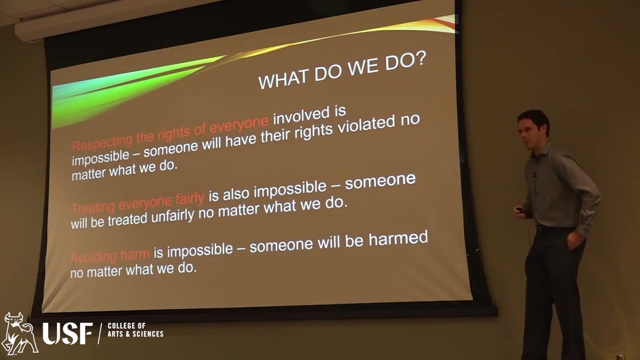 in the present who really need your political assistance and really need some other place to live. Phil Caparro's got a recent book where he explores this argument at great length. So what do we do in some of these situations, In this overall puzzle we've put ourselves? 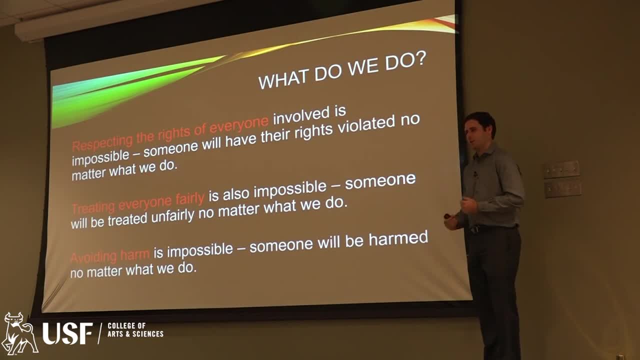 Because some of the moral things that we're taught when we're younger don't really work well here. You might say: well, I want to try to meet every you know, in case there are no rights violations occur, But you're screwed either way. 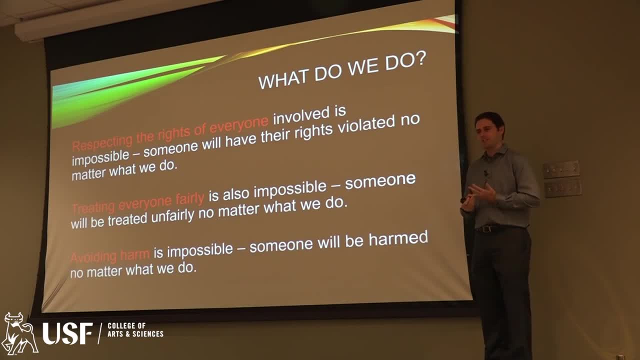 There are going to be rights violations. It's just the nature of the game. You might say. well, I don't want to try to avoid causing harm to anybody, But it's a given that somebody's going to get harmed somewhere in this overall process. 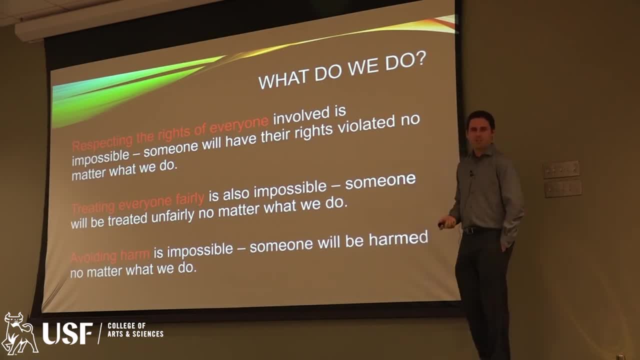 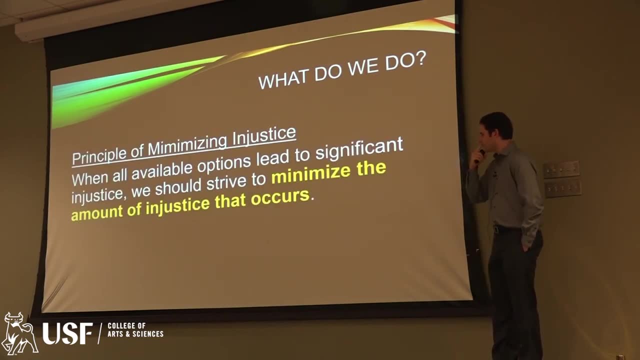 You might try to treat everyone fairly, But that's also impossible. Some people are going to get the short end of the straw. It's just a matter of who it's going to be and how many of them there will be. So here's the principle I propose for operating under these conditions of moral tragedy. 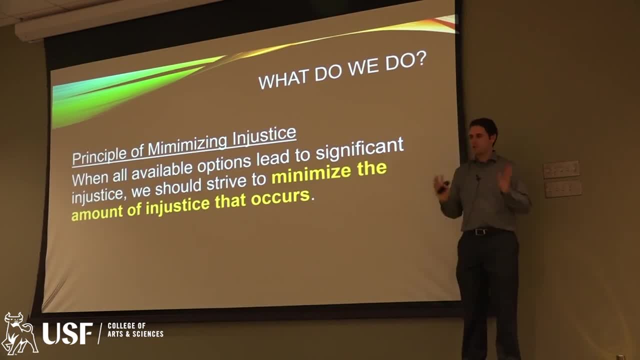 Why don't we try to minimize the importance of moral tragedy? Why don't we try to minimize the amount of injustice that occurs? We know there's going to be some that happens. There's going to be a lot that happens. Let's try to get less of it than what we would have had otherwise. 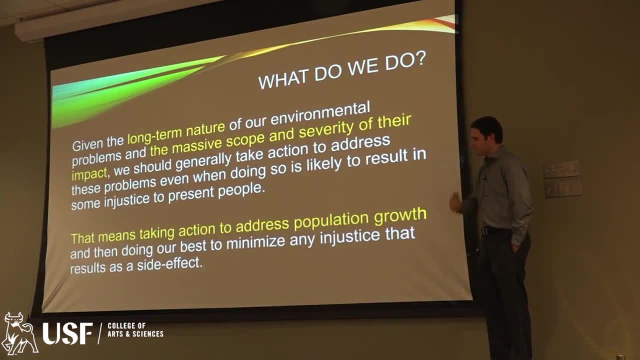 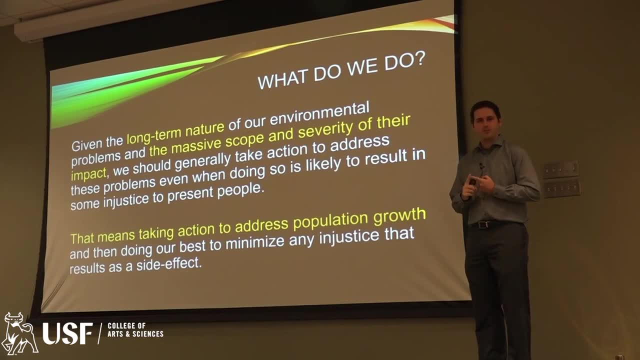 And so what does that mean in practice? There are three characteristics of our current environmental problems. They are very long term. Biodiversity loss can take millions of years to recover from Climate change. the CO2 will be in the atmosphere for thousands of years. 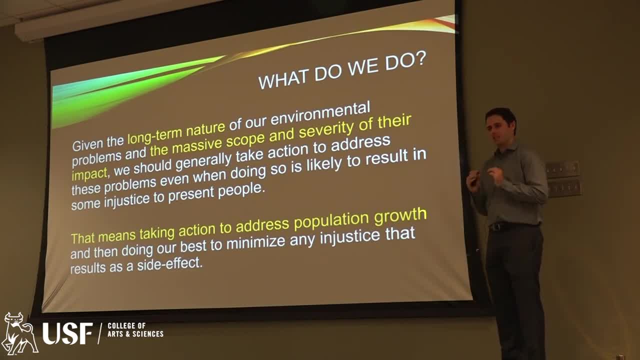 They are massive in their size and scope, affecting billions of people all around the world, And they are also very, very severe, because the impacts that these people will have will, in some cases, cause them severe suffering. In other cases, they'll just die, perhaps in a severe weather event or something like that. And in some cases they will have to relocate, have to uproot their entire life. So if you live on a low-lying coastal island, for example, your nation will literally be swallowed up by the ocean. There are already a couple of places in Kiribati and Tegulu where this is happening. 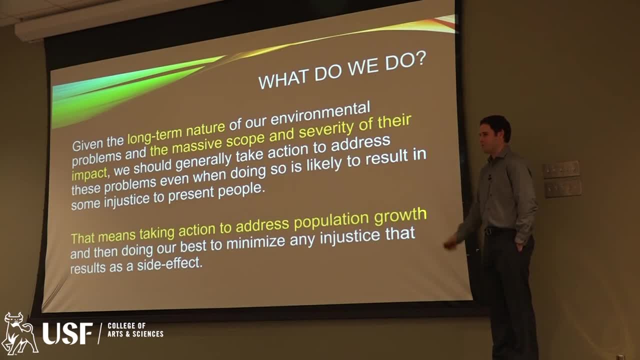 And these people are trying to mass immigrate out of their current situation. And so, given that, and given that I don't think there's any reason to prioritize, to value the life of someone in, say, 2018 over someone born in 2050,, I think that, in most cases, 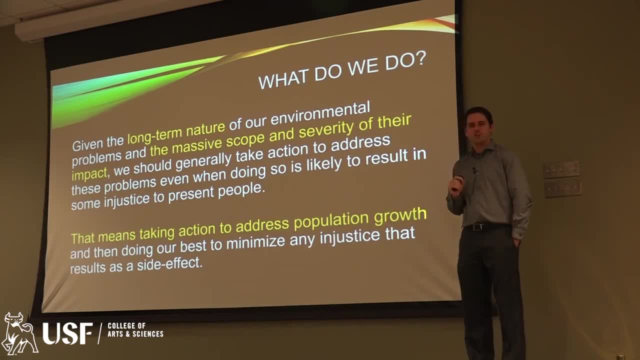 even if you're not going to be able to do that. you're not going to be able to do that, You're not going to be able to do that, There are going to be some resulting injustices. We've got to do what we can, what's available to us, to try to solve these problems. 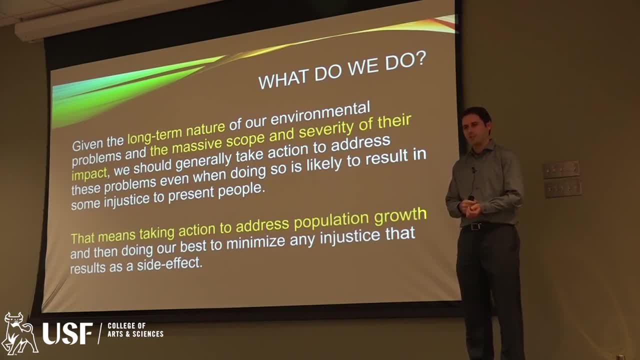 And that means taking population growth seriously And that also means foreseeably causing some unintentional injustice along the way. We'll do our best to minimize it, obviously, But if we don't do this, it'll be worse. The outcome will be worse if we do nothing than if we do something. 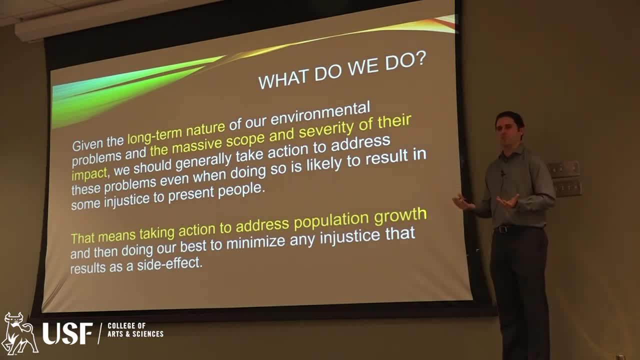 And since we're choosing between two bad outcomes, I think that's what we are more or less left with. So, in short, we've got to do something about population growth. It's going to be messy. There will be things that happen unintentionally, that are bad and that affect certain people. 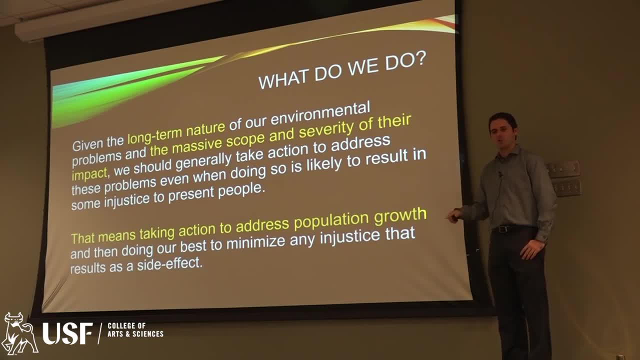 But not doing something about population growth will adversely affect an even larger number of people, and often in an even more severe way. So that's just kind of that's not a pleasant picture. I apologize if that's like basically the last slide and we're ending on a very compressed note. 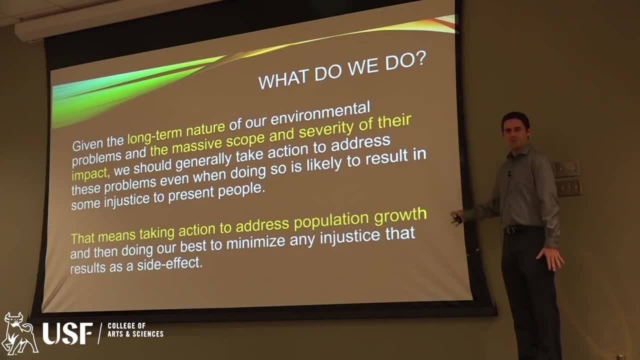 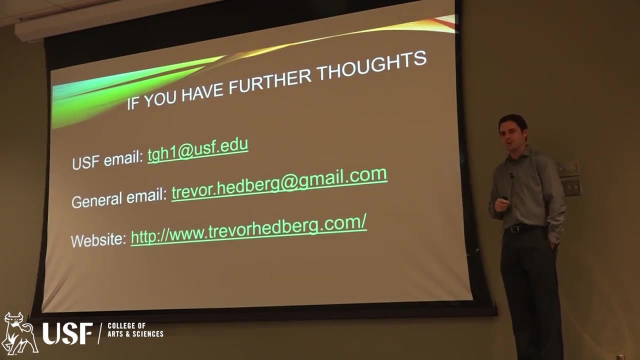 But I think this is a reasonable appraisal of our situation. It is not a case where there is a neat and tidy solution. There are only messy solutions, And so we try to clean up the mess as best we can. I'll also close by leaving my contact information up here if anybody has questions about this talk. 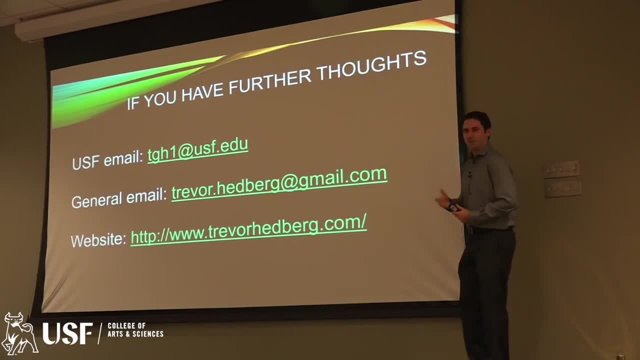 that I think you're not able to track me down later on. If we have time for questions from the audience, I'll take those now as well. So Kind of like in the country of the US, our system is mostly consumer-based. 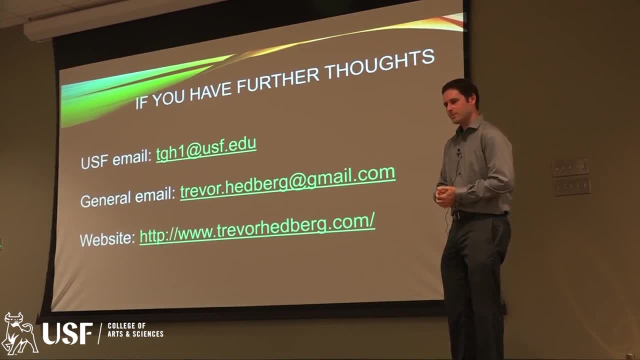 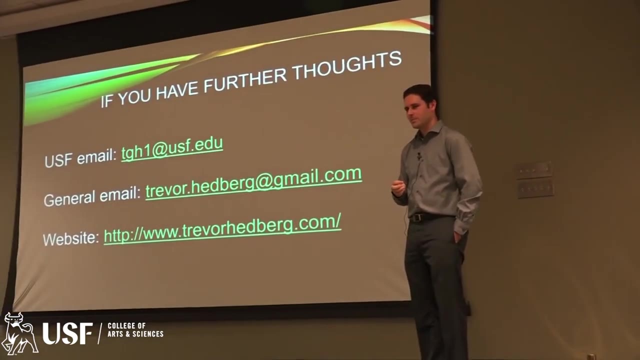 How would we kind of change that system to where it's less consumer-based? Because, going back to what you said, those incentives to allow tax breaks for people to go to school, it seems like the reason it's hard to change it, because it seems like there's more incentive to have more kids Because it will also be driving up that consumption. Yeah, So economists love population growth because there's more people spending money and contributing to whatever economy you have. And they also often will say things like people are the ultimate resource of ideas and innovation. 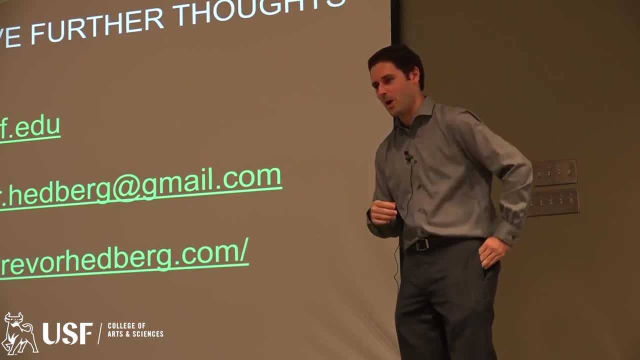 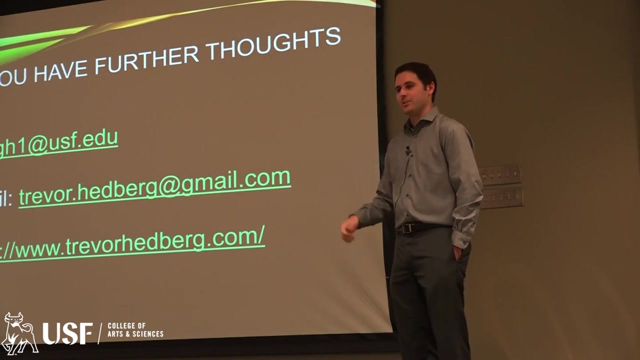 and so on and propose technological solutions to some of these problems. I'm a lot more skeptical about those kinds of prospects than they are. As far as how you initiate that sort of shift, we have to convince people, and there is some literature to this effect. we have to convince people that perpetual growth is not the route. 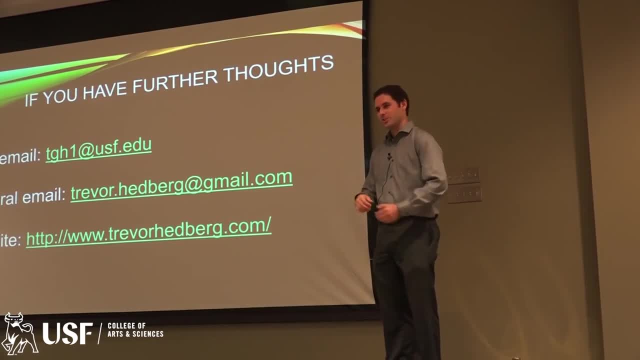 to human happiness, which is a tough sell, But there is some fairly compelling evidence that is true, that just an increase in GDP, for example, is not automatically correlated, past a certain threshold, with increases in happiness. Yeah, And so we have to get people to eventually say enough is enough and be willing to be. 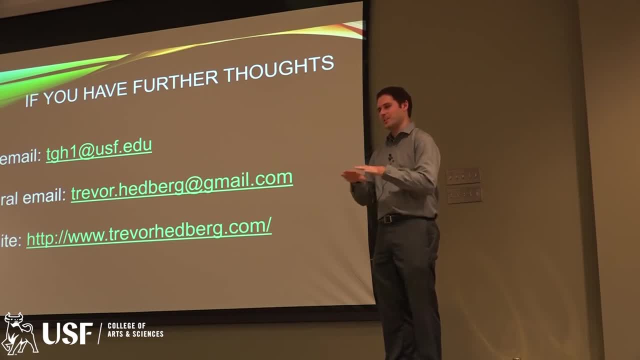 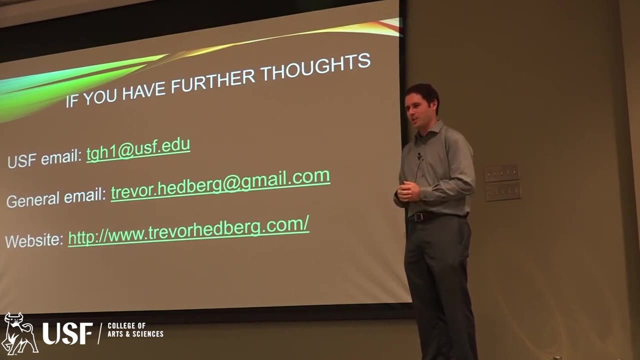 satisfied with essentially maintaining some sort of threshold of economic gains, as it were, rather than trying to get as much as possible indefinitely into the future. How we do that is very difficult and complicated, which is one of the reasons why we're in this. 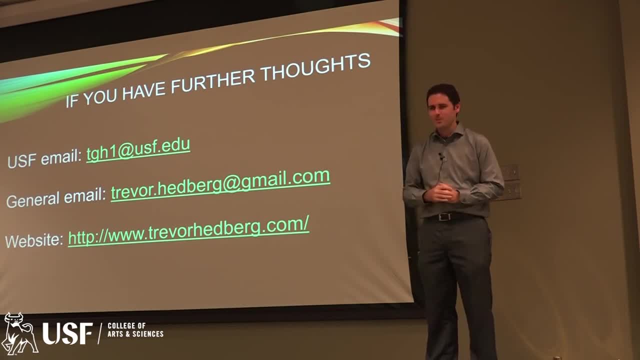 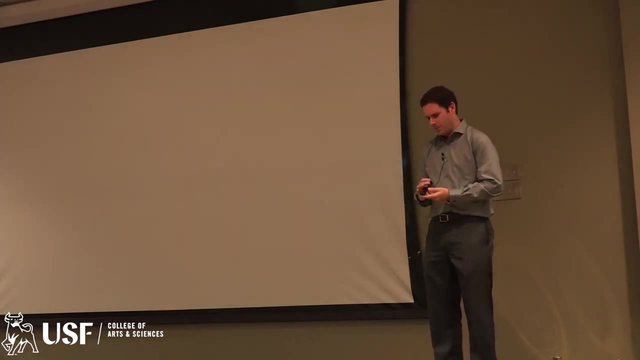 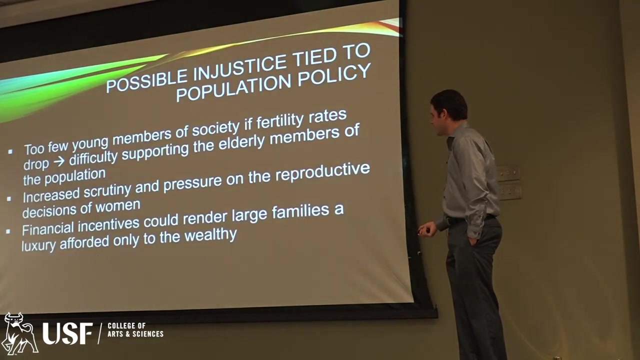 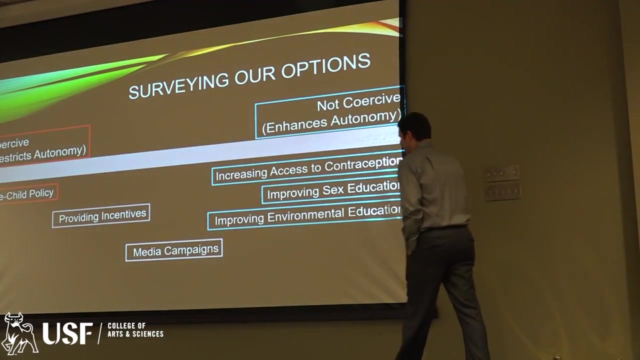 mess in the first place. So media campaigns, I would say. well, it may depend a little bit on the content. so the way I tried to graph it was to capture that idea. So I tried to put it more towards this side than like kind of towards the middle. but 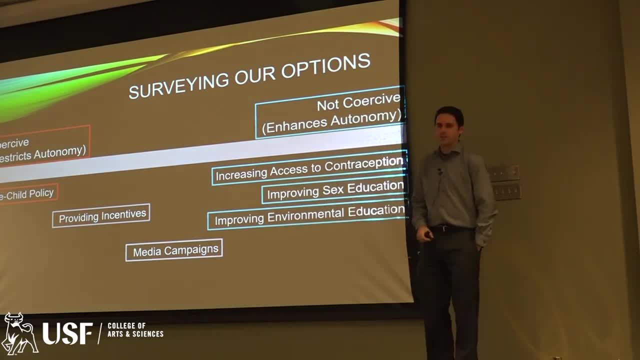 more towards the middle, So a little bit more towards this side. I think that media campaigns are less, much less at risk of being autonomy-restricting than incentives will be, And I think, as I said, in some cases I think they can be autonomy-enhancing. 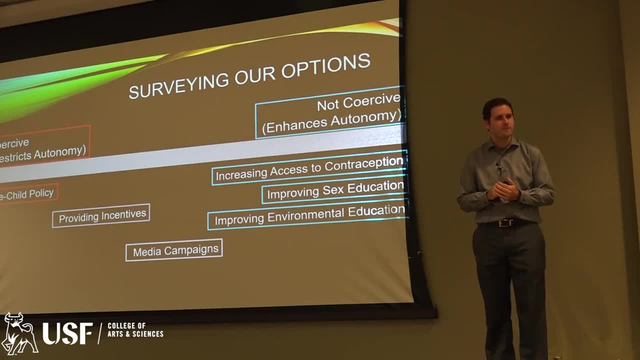 So in your early equation of environmental impact, you chose to omit wealth and large wealth-moving entities, Right? So in your earlier equation environmental impact, you chose to omit wealth and large wealth-moving entities. So in your earlier equation of environmental impact, you chose to omit wealth and large wealth-moving entities. 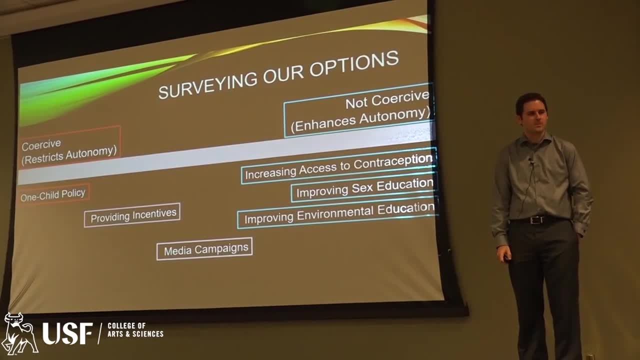 Ignoring that in your early equation does not detract in nuance from things that are affected by that, like large resource hoarding and the access to education that that would result in large population growth. If you can't afford the education, you can't reach the education. you can't get the education to know better. 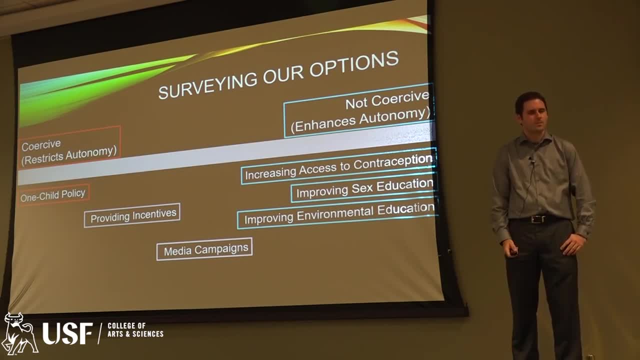 So if somebody is hoarding the money and somebody is hoarding the education and hoarding all the access to medical services, especially in over-exploited countries, do you feel like that might lose, especially when you're discussing the eugenics and the social redefinition? 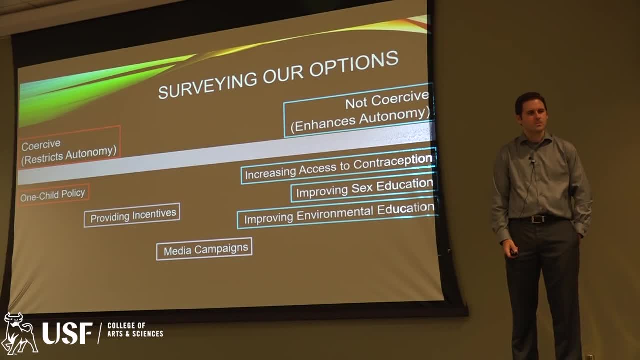 I mean definitely you have a social redefinition of parent or family is essential and education is essential for the restriction. But large moving money entities are by far more carbon-consuming And our choice of changing a baby to one child or not having a child, having a child 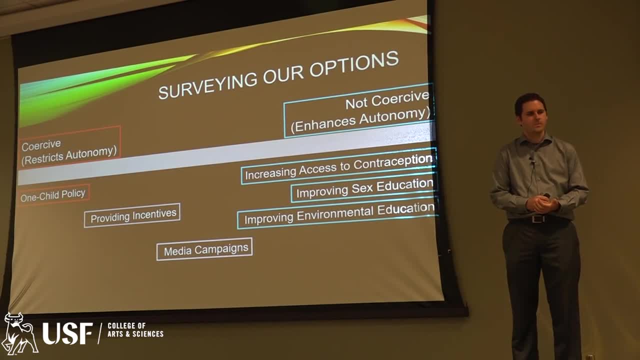 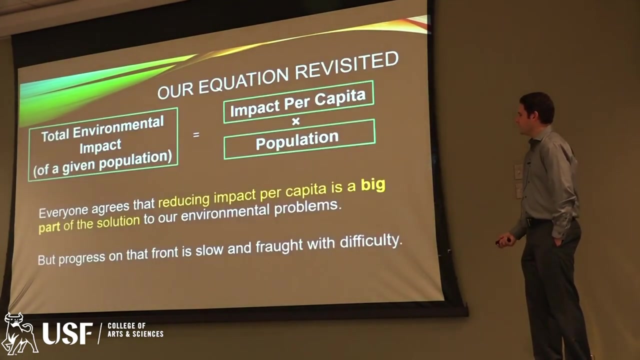 really makes very little impact based upon one large and wealth-moving entity. So how does that impact your population equation? How do you define the concept of wealth and large wealth-moving entities? Well, so I try to take that into account in the parenthetical part here. 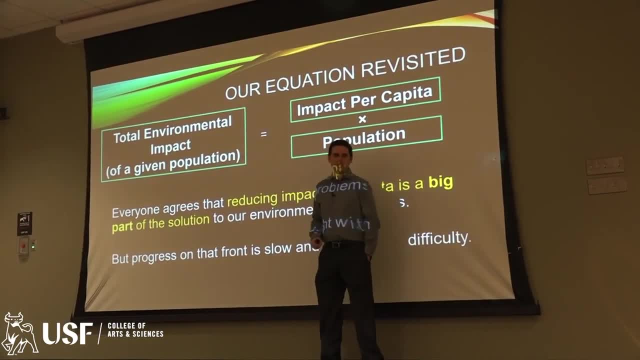 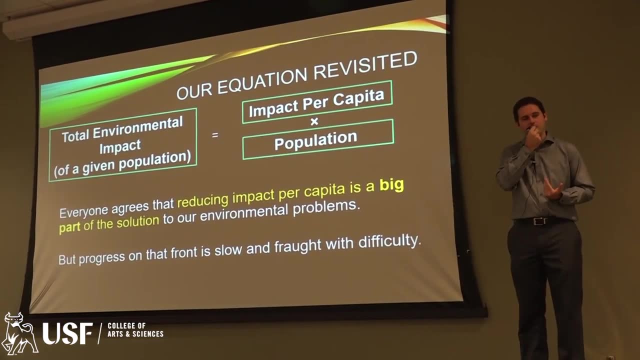 which is that so you can break this down, say, into total normal impact like other given population. You could break this down by country, for example, and you could look at because obviously a person living in the United States has a much different per capita impact. 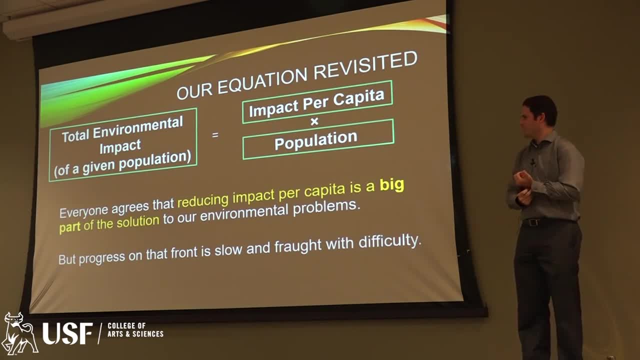 So you could look at, because obviously a person living in the United States has a much different per capita impact than a person living in Africa. Now, I didn't have time to get into this in this talk, but one of the significant factors I think might speak to your point. 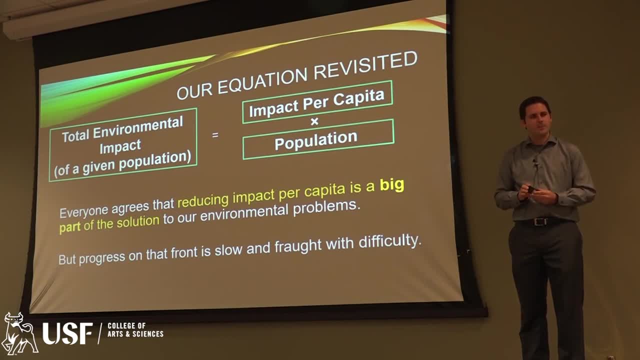 is the fact that I don't think it will be prioritized. I think the policies we're going to try to pursue in different places are going to be different and I think it will be prioritized to be different. So Travis Reeder has a recent book on this topic, for example from Springer. 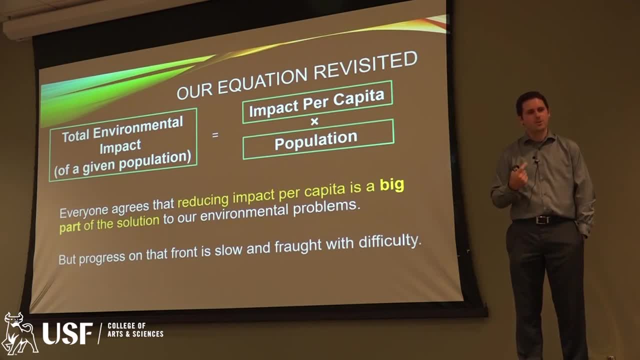 where he argues that the primary people who need to be concerned about restricting appropriation, even though countries, even though countries like the US and Western Europe- have lower fertility rates, it's still them, because the rates of consumption are just so much higher. 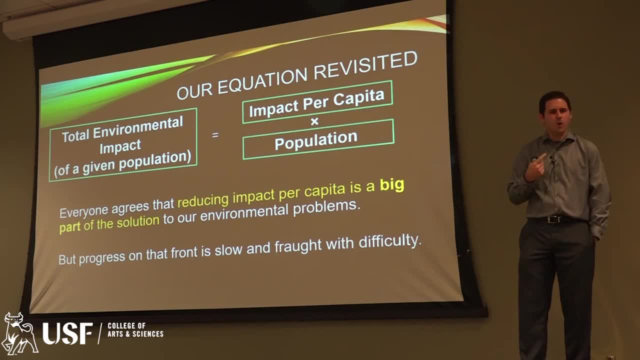 So you can call it with statistics like: one additional American child is the equivalent of, say, eight children in India or Malawi, or something like that. Although I think you mentioned something about- I don't know if this necessarily speaks to your point about- 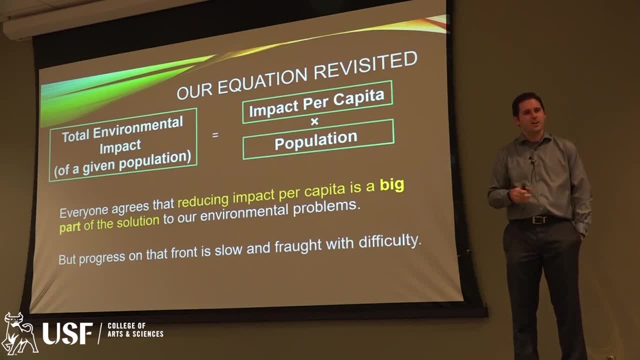 I don't know if this necessarily speaks to your point about. I don't know if this necessarily speaks to your point about large wealth holders. It doesn't necessarily. I was wondering if one American child was not going to displace the climate change and resource change that Coca-Cola is going to do. 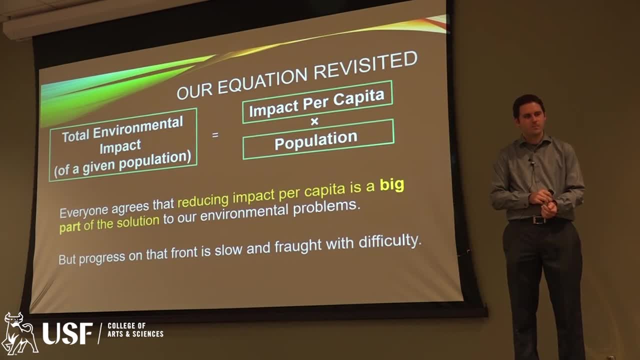 and Coca-Cola is a globalist. So that's how I'm wondering how the population and restricting population, especially when, as you have pointed out, wealth influences a great deal of your labor, You have problems with incentives etc. or a lot of the injustices are based on inequalities or hierarchies regarding wealth. 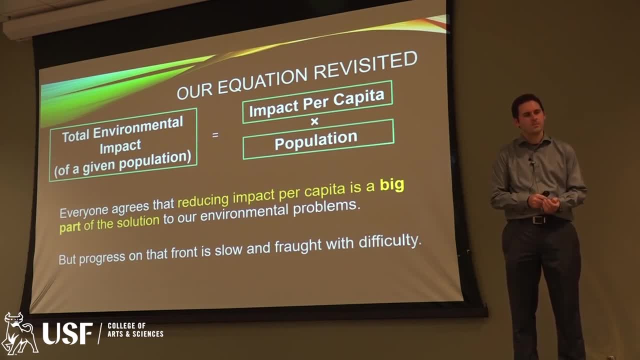 If you don't have wealth in the equation to begin with, and understanding the large wealth removing entities, then how do they equate? That's my question. Okay, So I'm not sure exactly how to reduce the formula that I've got to capture the environmental impact of Coca-Cola. 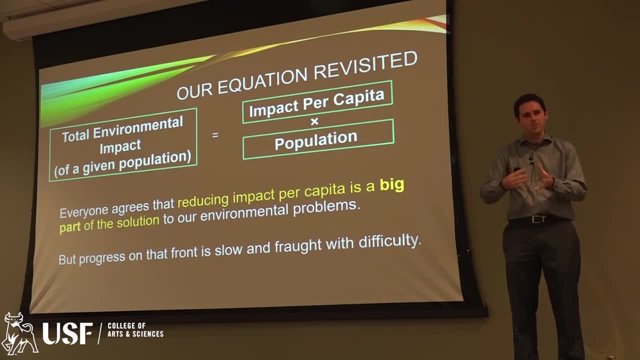 or some other corporation that can't just reduce the number of members it has, or something like that. I imagine there are some sociologists who have tried to do that with something like iPad. I'm not sure exactly how well it could do with something like that either way up. 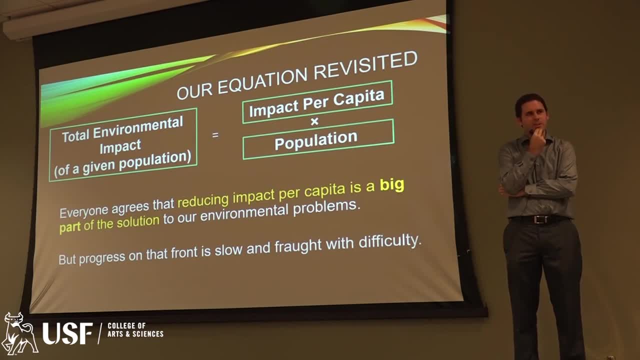 hand, But I think that the challenge of essentially dealing with those kinds of entities strikes me as something that's important and worth tackling and part of reducing consumption patterns more generally, but probably lies outside of the scope of what I'm addressing here. All right, Thank you very much, Trevor. Thank you very much.